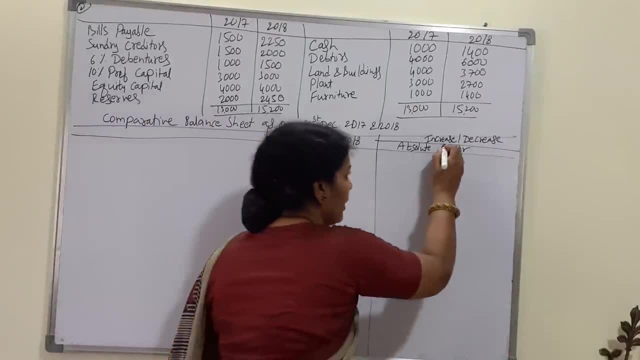 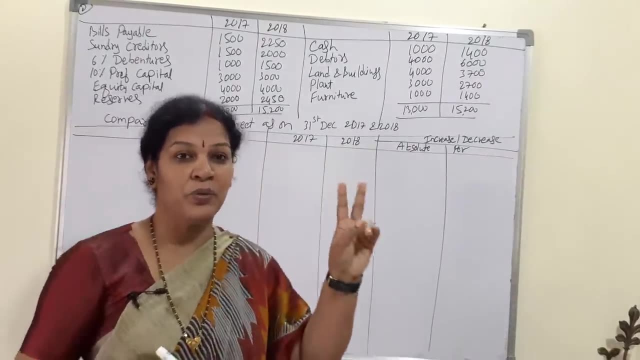 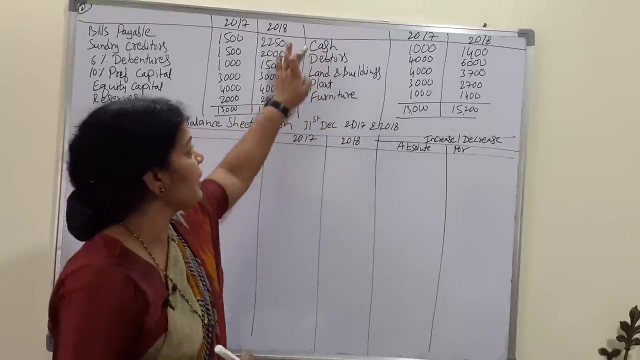 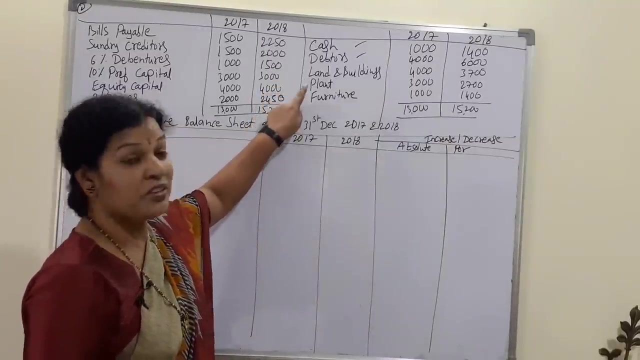 Increase or decrease. That's in absolute and percentage wise. So first, what we'll take here, Assets. Assets we are going to divide into two parts. One is current assets and fixed assets. Right Now, assets, if you see cash debtors. These two are current assets. Next, land and building, plant furniture. These three are fixed assets. That we'll mention it here. 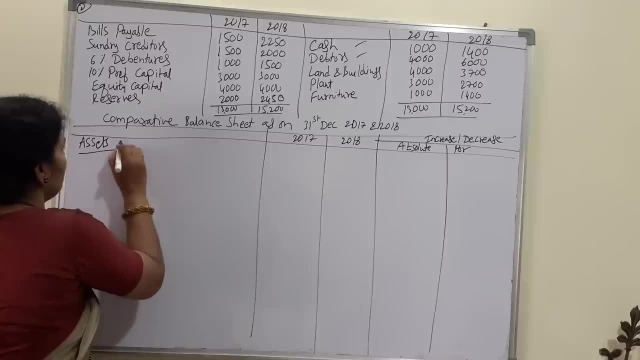 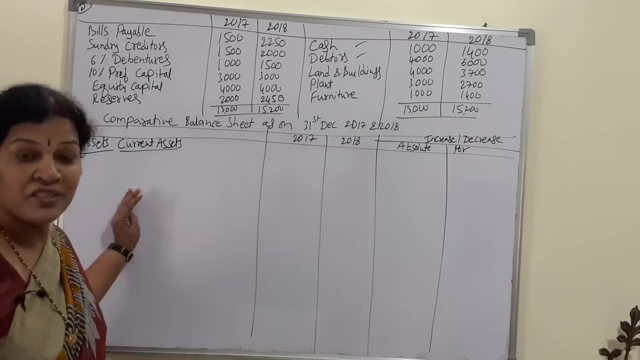 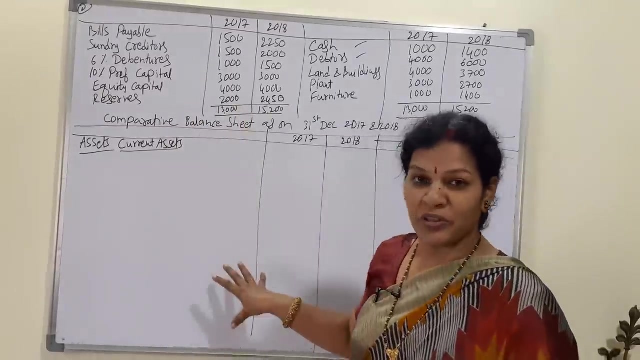 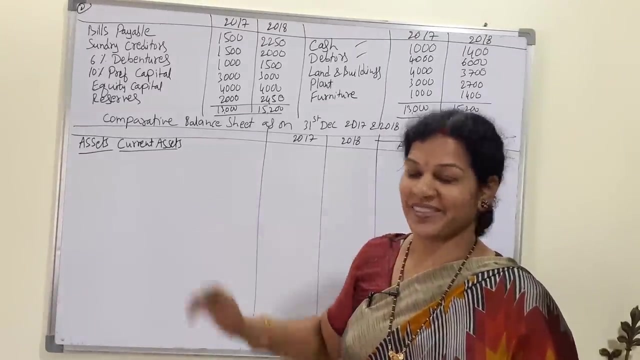 Assets- Current assets- Space is less Generally, we'll write assets under that: Current assets. Under current assets we'll be mentioning, because the board is very small. That's the reason I'm writing just beside Now, current assets. also. I'll start writing here only because, to save the place, 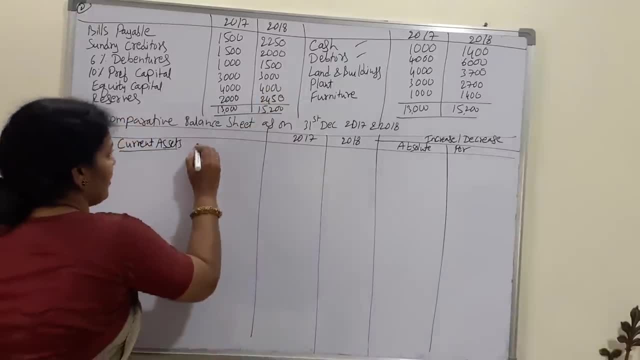 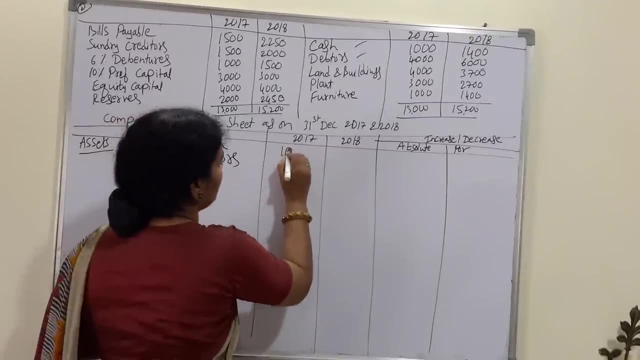 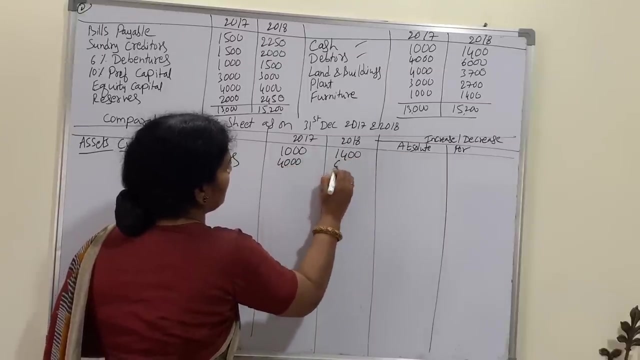 Current assets. What do we have? Cash and debtors? Cash is 1,000 and 1,400.. Debtors 4,000, 6,000.. So these are current assets. So we'll write here: total current assets. 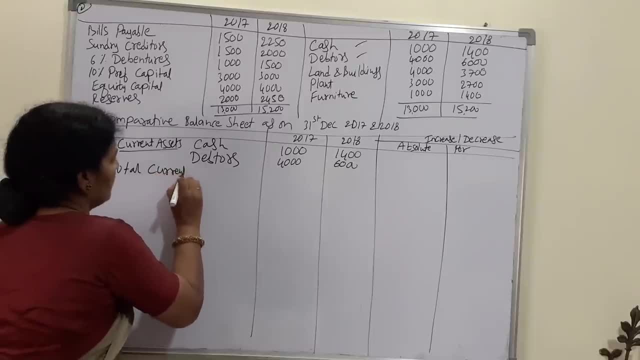 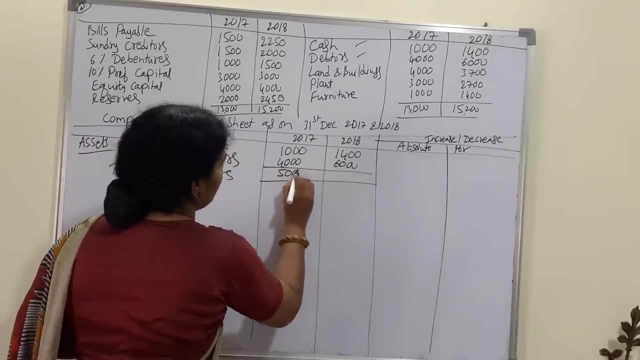 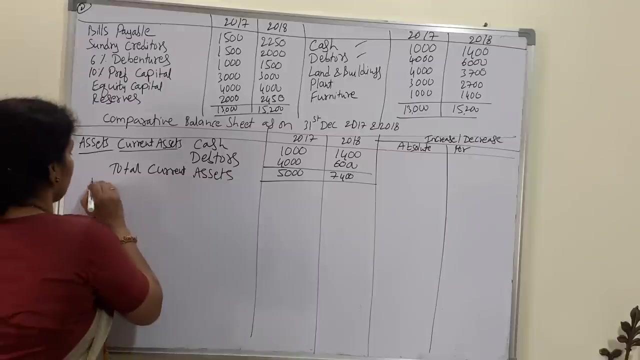 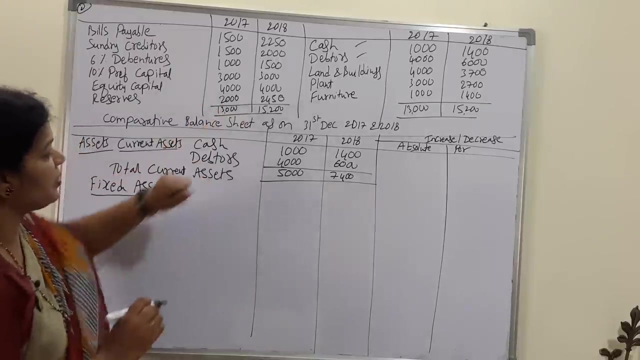 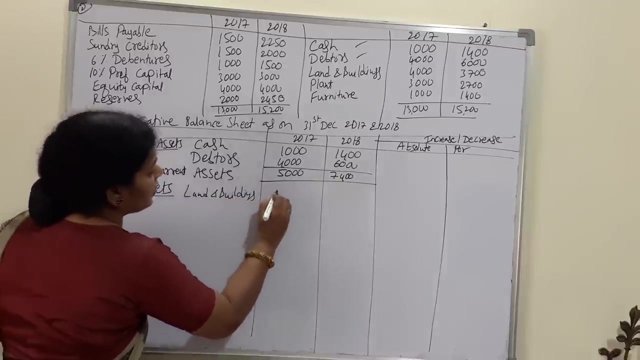 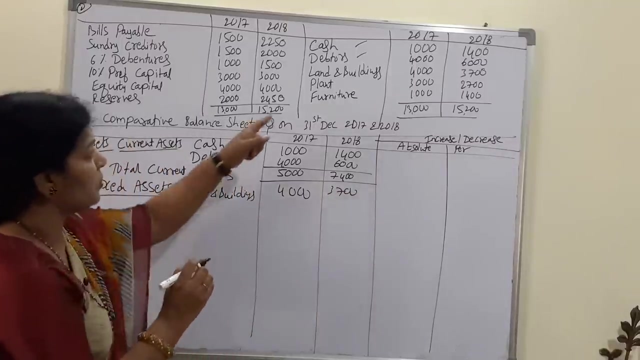 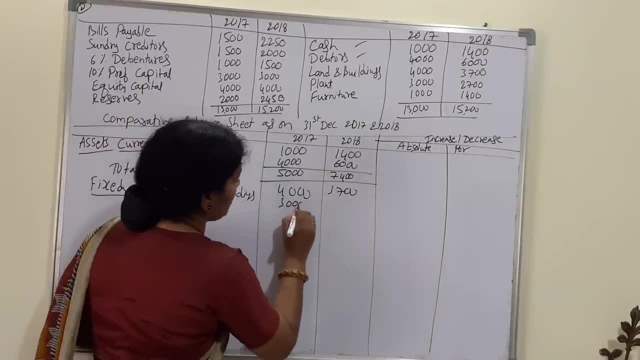 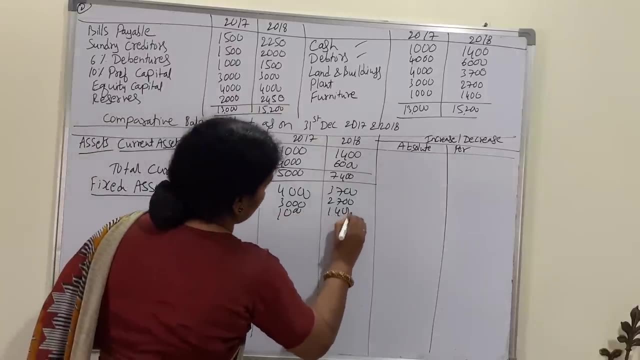 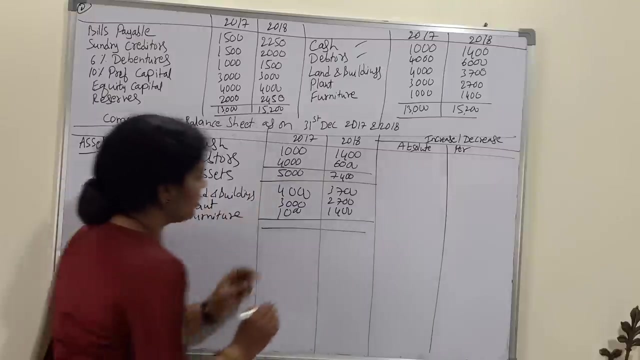 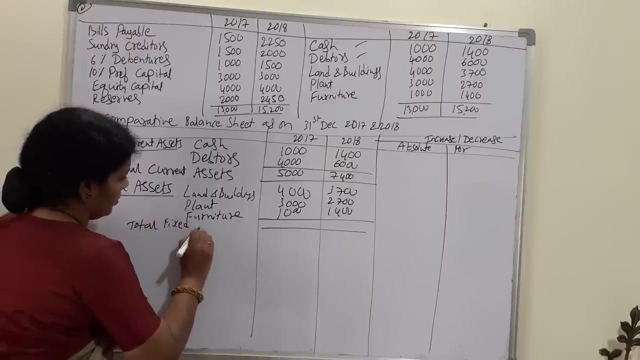 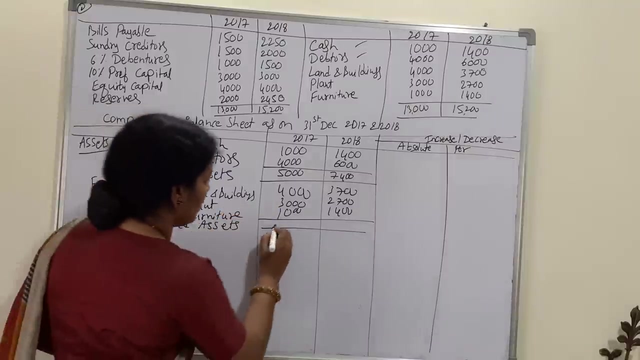 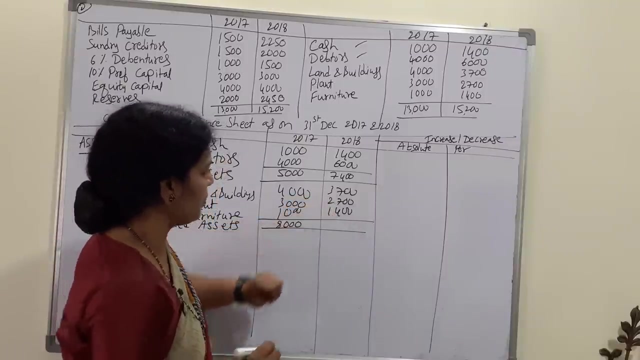 1,000.. 3,000, 2,700.. Furniture: 1,000 and 1,400.. So this is fixed assets, total fixed assets. Total fixed assets are 3 plus 4, 7,, 7 plus 1, 8.. And here it comes 14,, 14 plus 4, 8, 18, means 6, 7,800.. 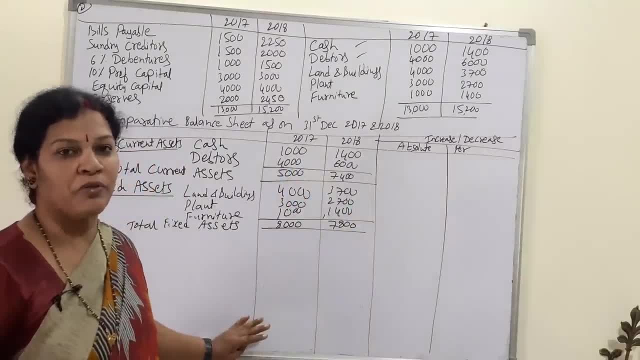 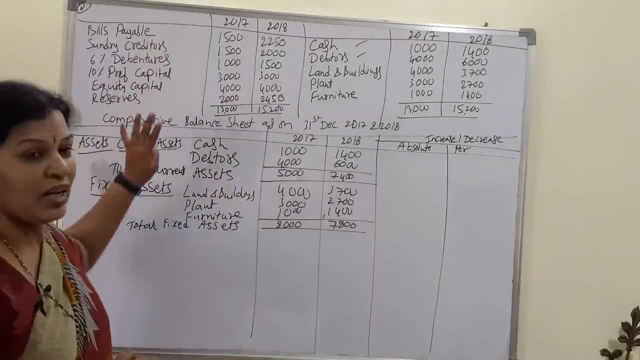 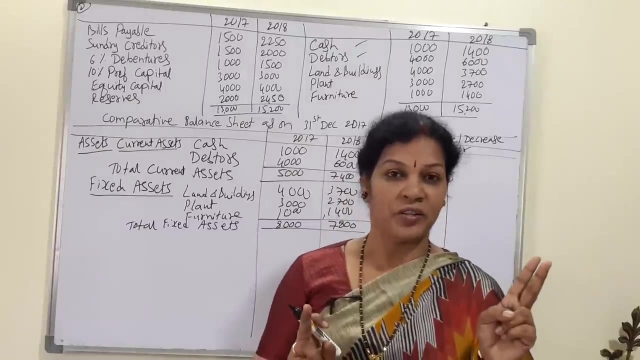 Increase or decrease percentage. we will do it later. First, we are writing the pro forma Now. this is about current assets and fixed assets are over. Assets side is over. Now coming to the liability side. Liability side: what do we write? first, Current liabilities. Second, long term debt, long term debentures. 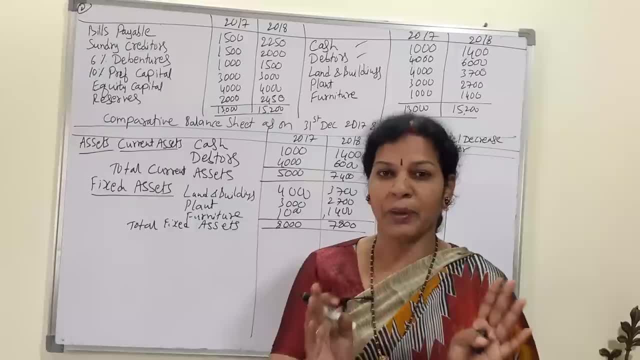 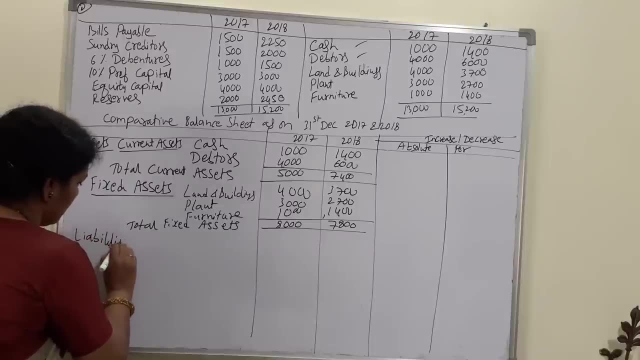 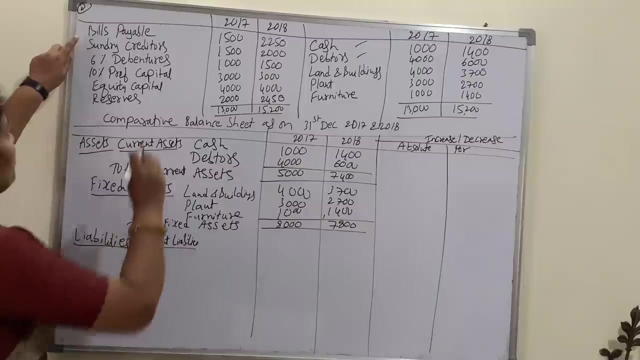 Third one, reserves and capital. Three parts will do it right. So liabilities, current liabilities Under liabilities. we will write current liabilities Under current liabilities. what do we have? Current liabilities bills payable creditors: Only two are there. 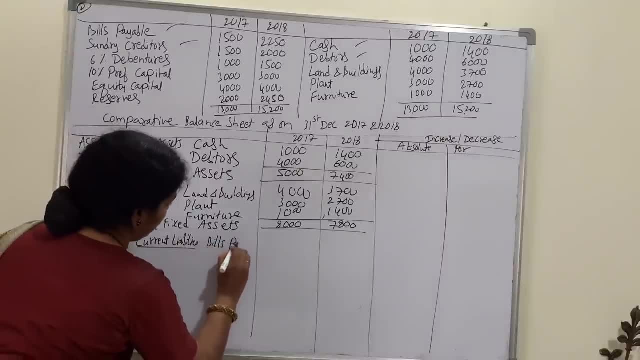 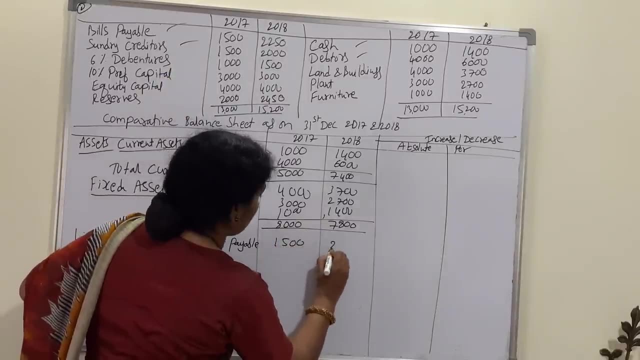 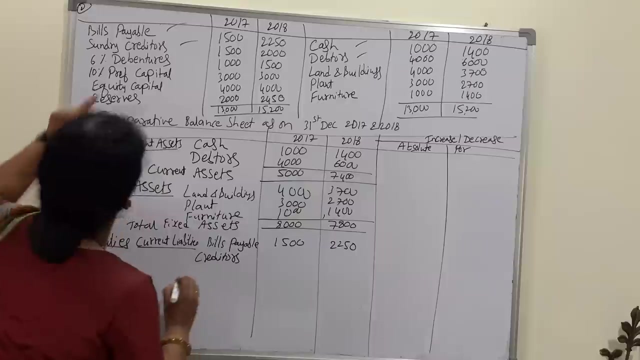 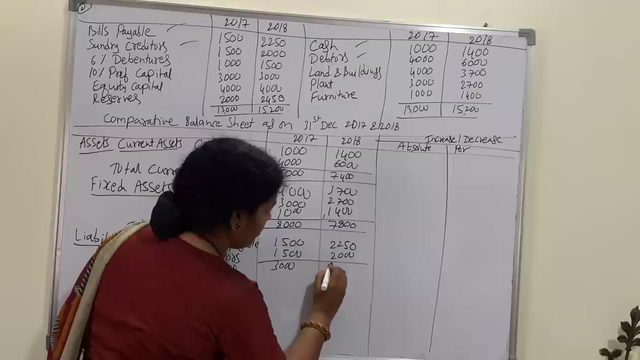 So we will write that bills payable: Bills payable: 1,500 and 2,250.. Then creditors: Creditors are 1,500 and 2,000.. So these are the total current liabilities. Total current liabilities are 3,000 and this is 4,250.. Next, after that, we will write long term debt. 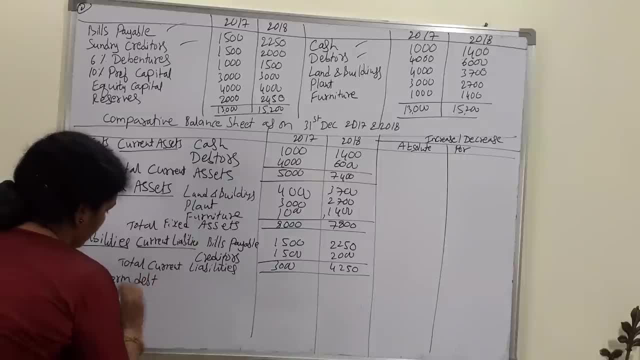 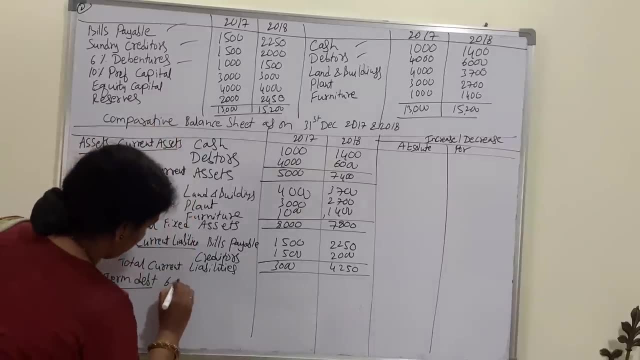 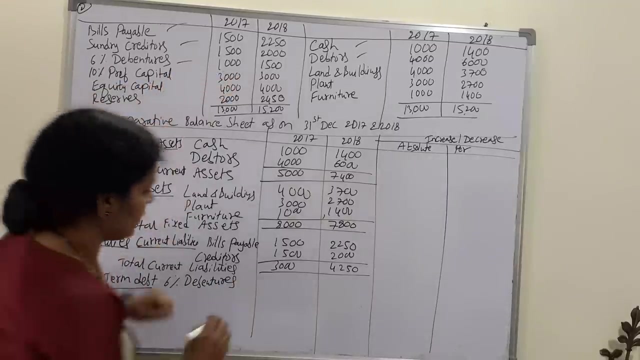 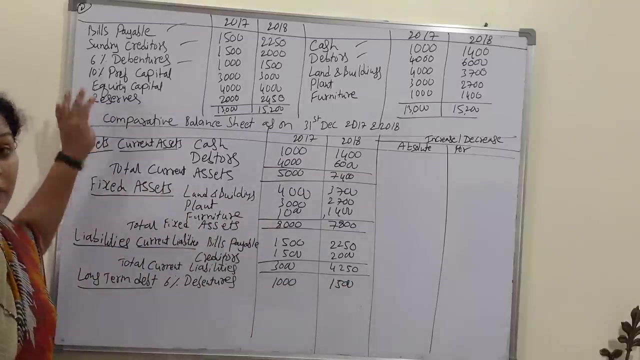 What do we have? Long term debt, 6% debentures Only this is long term debt, 6% debentures. This is 1,000 and 1,500.. Then after that we will give a side heading. that capital and reserve Capital is here preference share capital. 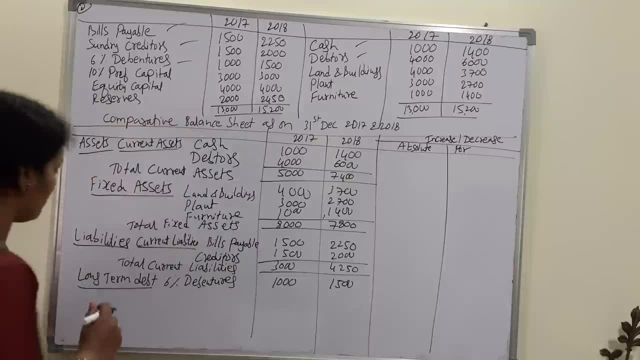 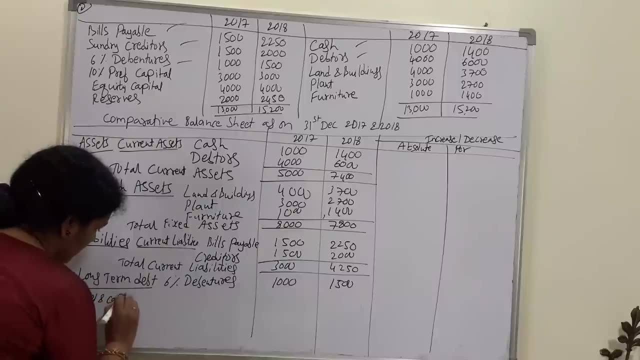 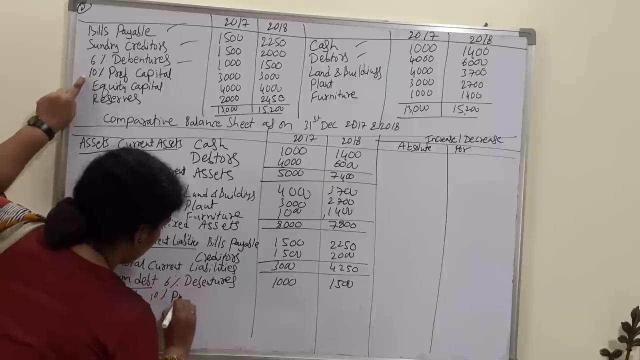 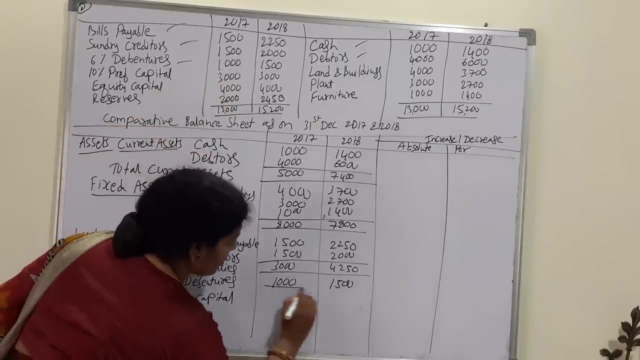 Equity capital. Both are capital and reserves, both together Reserves and capital. Under this first, preference capital, 10% preference capital: 3,000, 3,000.. This is over 3,000, 3,000.. 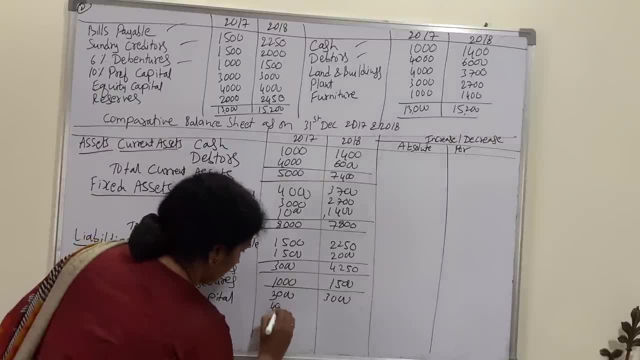 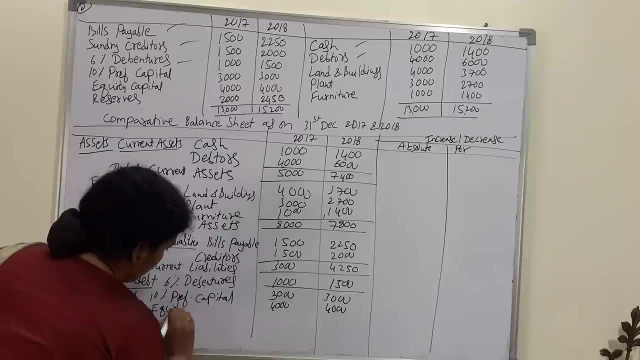 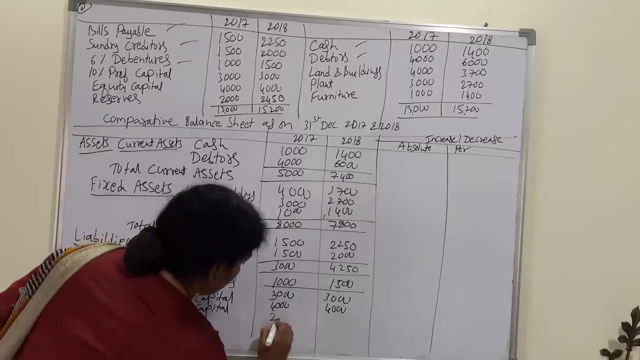 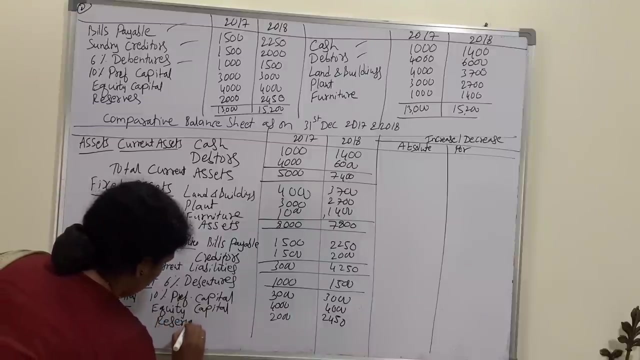 Next equity capital: 4,000, 4,000.. Equity capital, After that reserves: 2,000 and 2,450.. Reserves: this is So. we will total up 3 plus 4.. 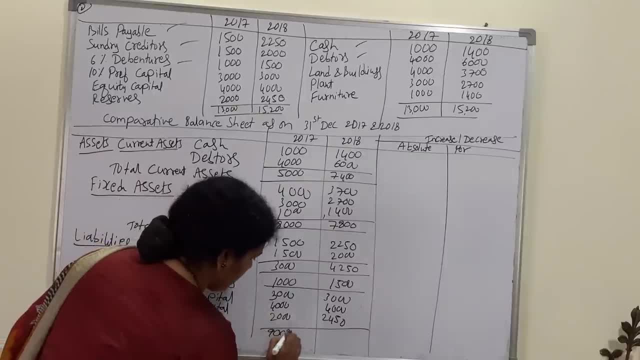 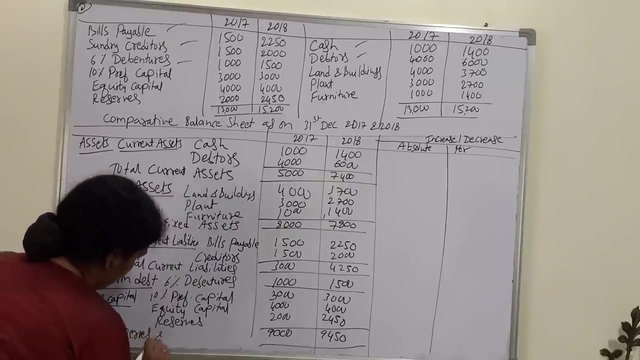 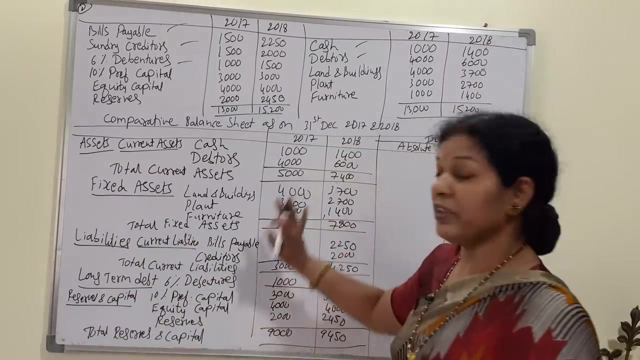 7, 7 plus 2, 9,000.. And here 7,000, 9,450.. This is total reserve and capital. So, like we have prepared the pro forma, Please remember quite easy and when you write it in the exam. 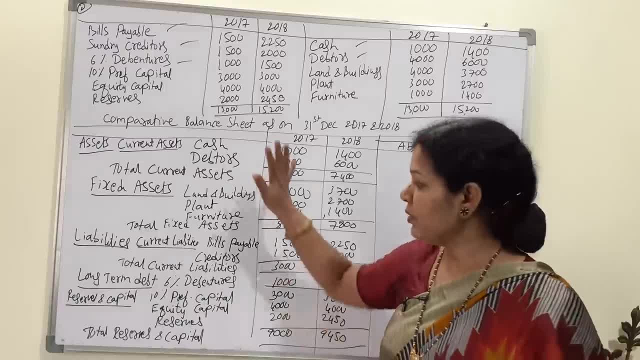 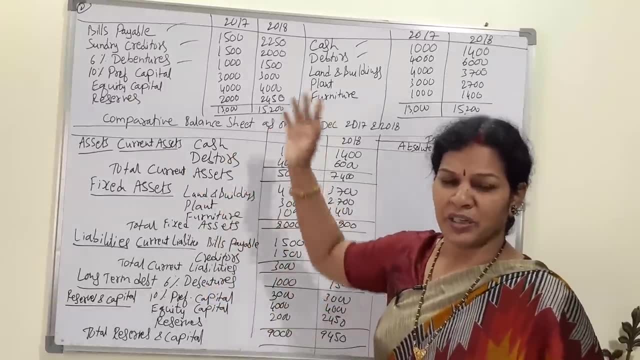 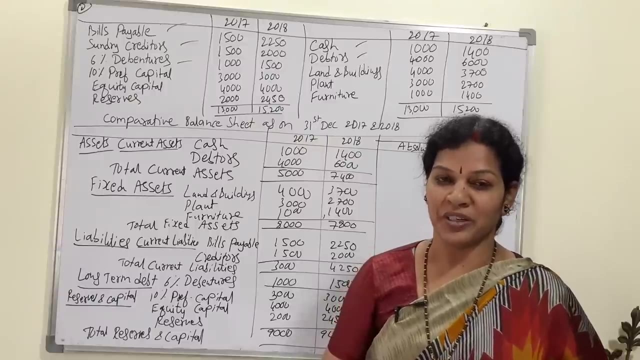 please use Free space comfortably. you can write neat handwriting and with scale. you can draw the table and debit credit and whatever it is, The pro forma has to be very neat and clean For the pro forma first impression the examiner is going to get. 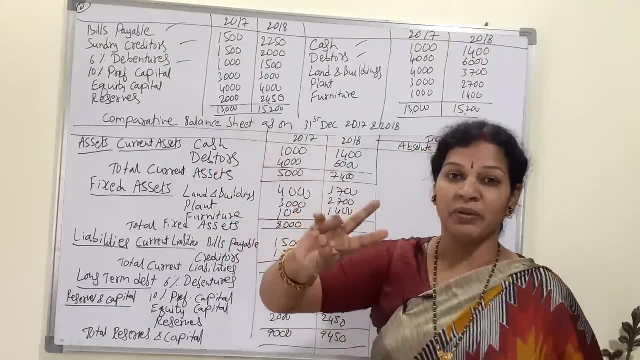 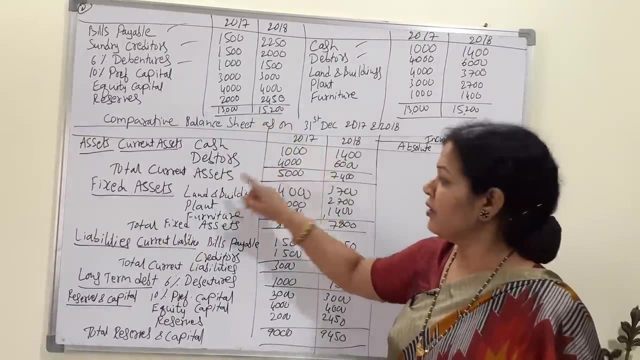 Now let me give you a recap what we have done here. First, assets are divided into one part, two parts: current assets, fixed assets. Current assets: we have cash and debtors return. total current assets, Then, after that, fixed assets. 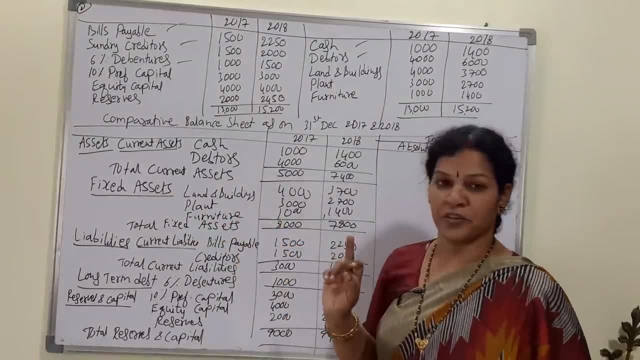 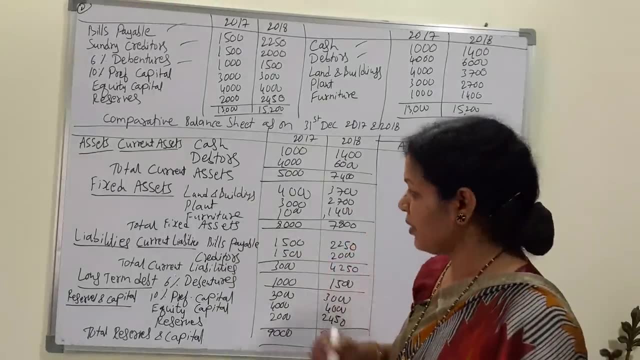 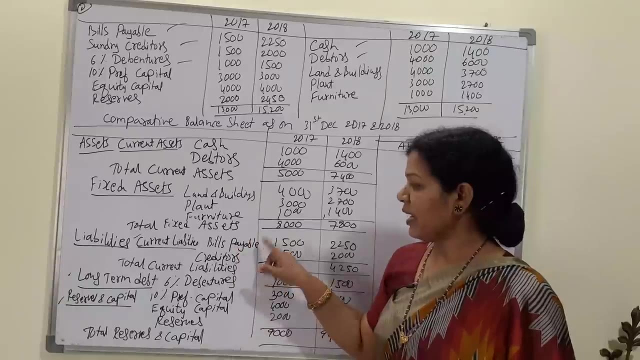 Fixed assets are here: land and building, plant and furniture, Total, total fixed assets. So this is about assets. Now coming to the liabilities, we have three parts. One is current liabilities, long-term liabilities and reserves and capital. Current liabilities: we have, as per the problem, bills payable, sundry credit hours. 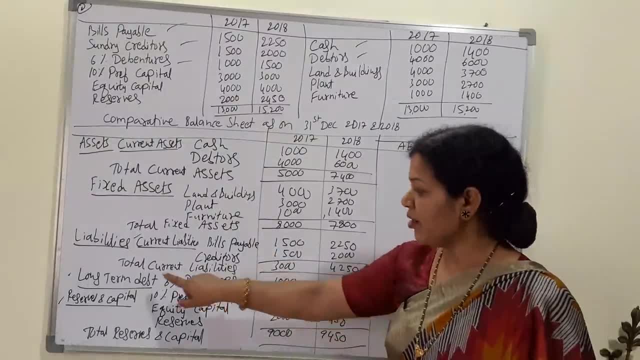 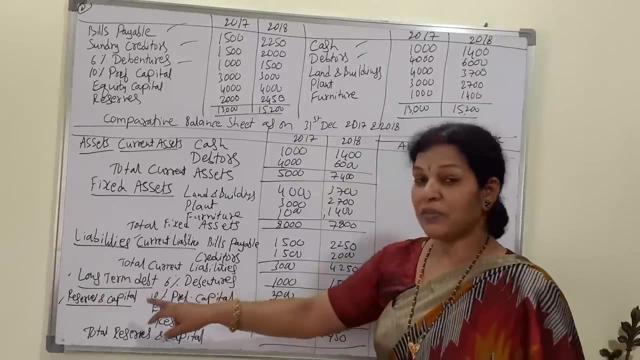 These two we have written. So this is total current liabilities. Next, long-term debtors: here we are having debentures, Debentures, long-term loan Debentures, loan debt. we call it then after that reserve and capital, we have preference capital and 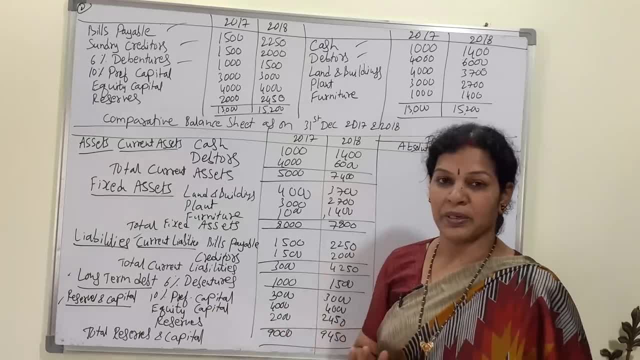 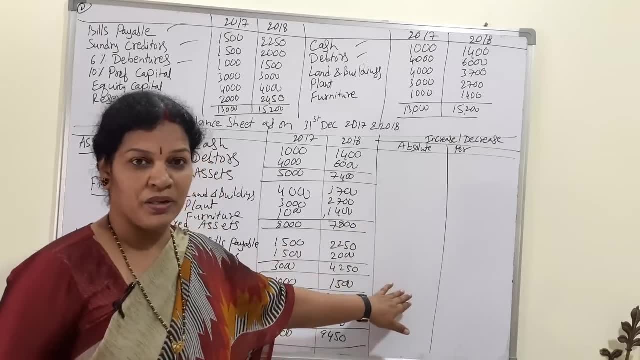 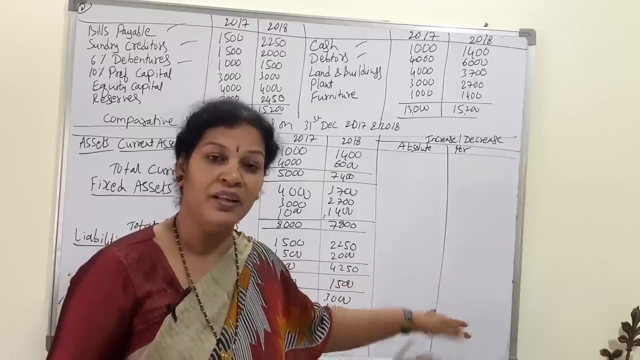 equity, capital and reserve. these three comes under the reserves and capital total it. so this is the pro forma. now, what we need to do, just increase or decrease will write and also percentage, same like previous income statement, comparative income statement. however, we have done in the same fashion. we are going to do so. first one is here: thousand to fourteen. 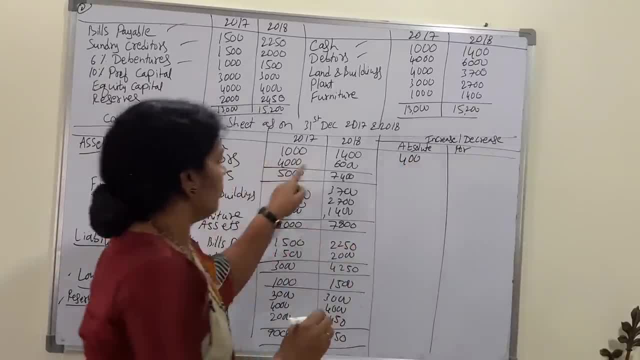 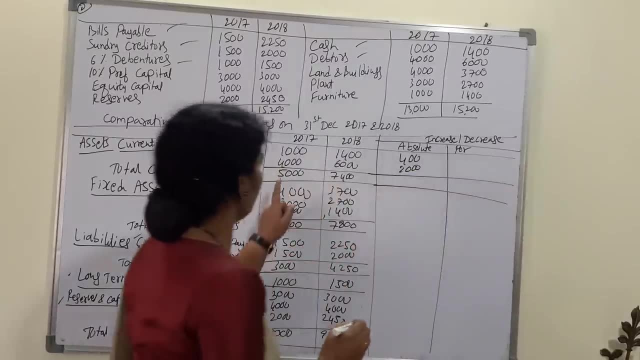 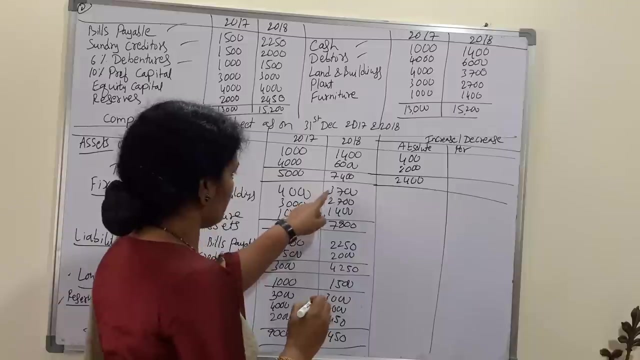 hundred means four hundred, increased four thousand to six thousand means two thousand, increased now here fourteen, two thousand, four hundred. next, this is three hundred, decreased three hundred. now here also three hundred. now here also three thousand to two thousand, seven hundred, three hundred. once again here it is decreased. 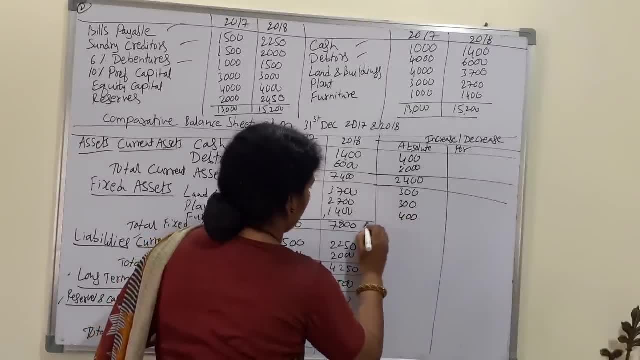 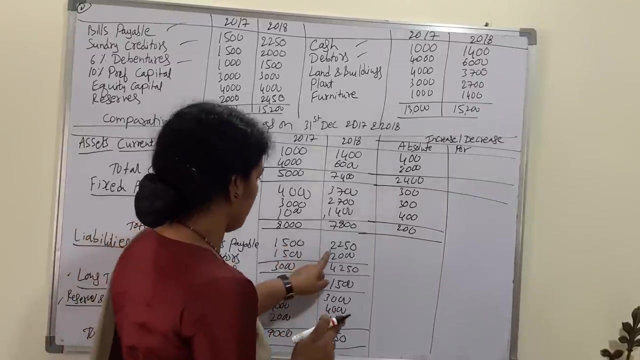 thousand to fourteen hundred four hundred. so here it is one thousand eight hundred, sorry, two hundred. only eight thousand to seven thousand, eight hundred two hundred. in the same way, fifteen hundred to two thousand two fifty means seven fifty here. fifteen hundred to two thousand two hundred, here it is three thousand to two thousand. 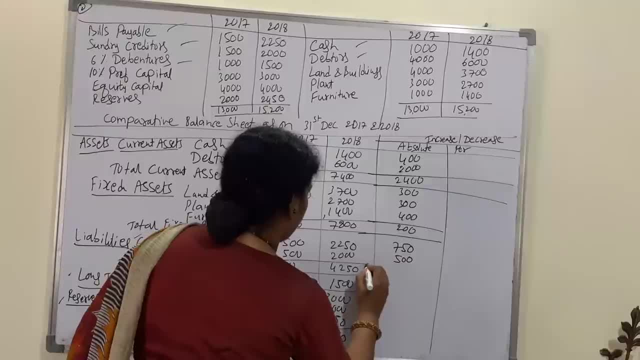 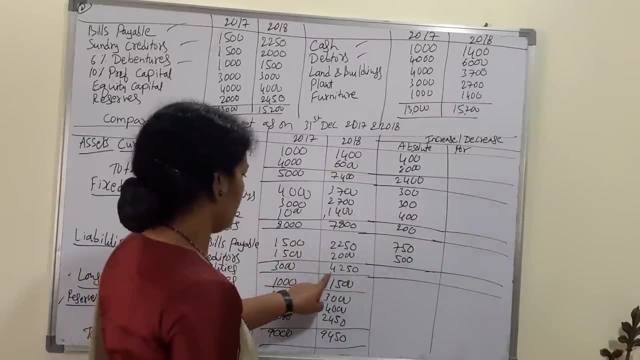 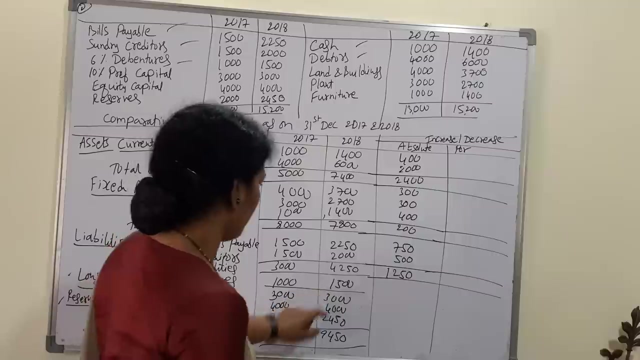 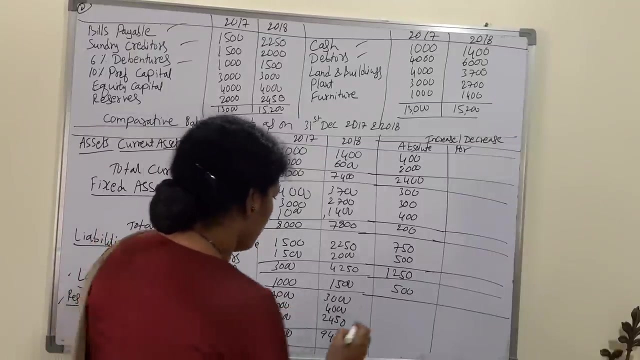 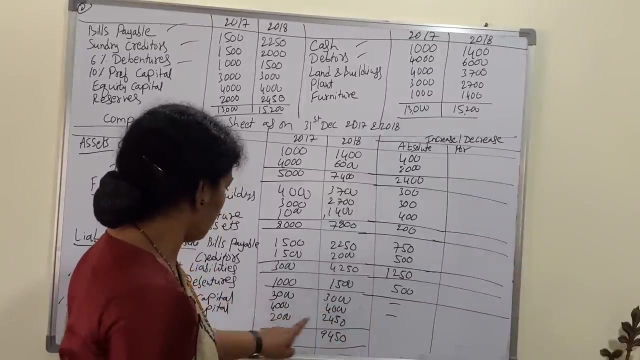 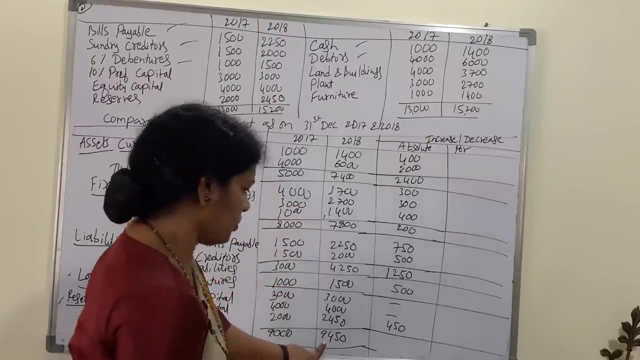 thousand five hundred. so this is one thousand two fifty. next debentures: 500 increased. next preference capital: no increase, no decrease. and the equity capital of four thousand four thousand, no, no difference. and reserves are two thousand to two thousand. four fifty means 450 increased. lastly, nine thousand. 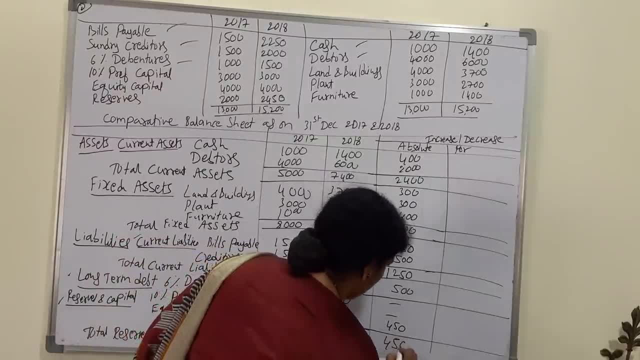 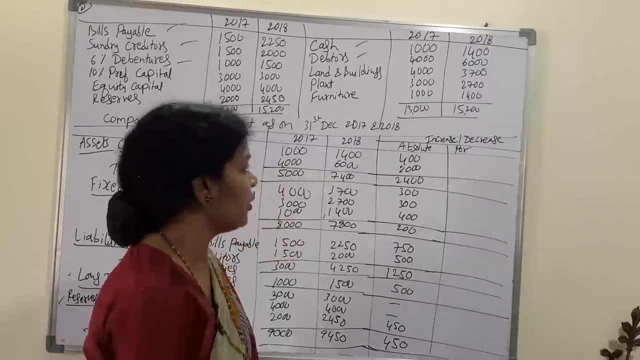 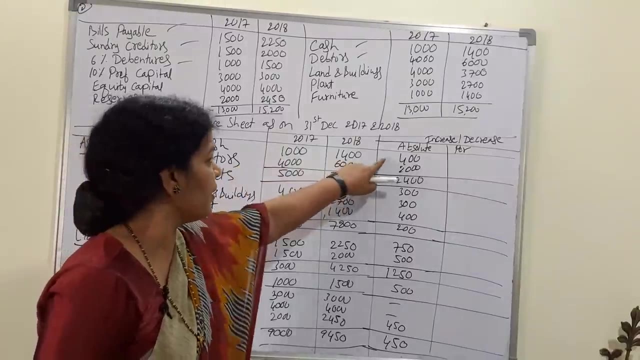 to nine thousand four fifty means 450 increased. so this is increase or decrease. we have written now what to do. calculation of the percentage. to get the percentage always remember: increase or decrease this amount divided by base basis 2017. 400 divided by thousand into basis 2017. 400 divided by thousand into: 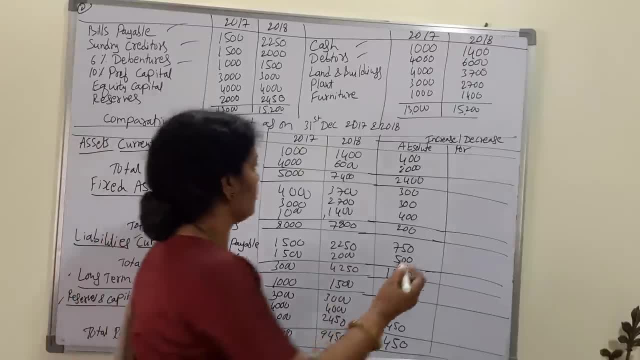 basis 2017. 400 divided by thousand into hundred. this 40%, this is 40% in the same hundred. this 40%, this is 40% in the same hundred. this 40%, this is 40% in the same way. all the amounts we need to calculate. 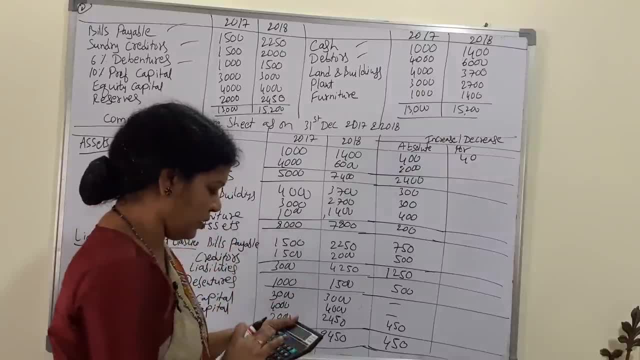 way all the amounts we need to calculate. way all the amounts we need to calculate. 2000. the second one is 2000 divided by 2000. the second one is 2000 divided by 2000. the second one is 2000 divided by four thousand. two thousand divided by: 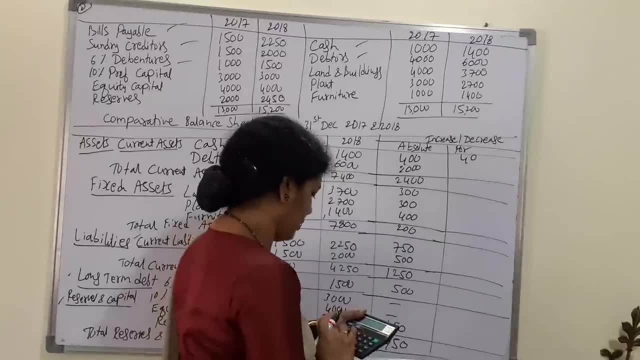 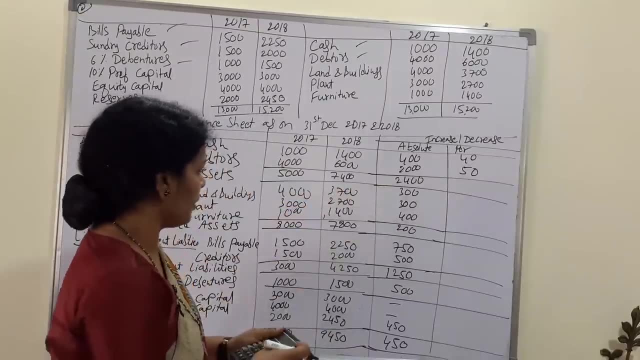 four thousand two thousand divided by four thousand two thousand divided by four thousand into hundred, it is 50%. next, four thousand into hundred. it is 50%. next, four thousand into hundred. it is 50% next to two thousand four hundred, to two thousand four hundred. 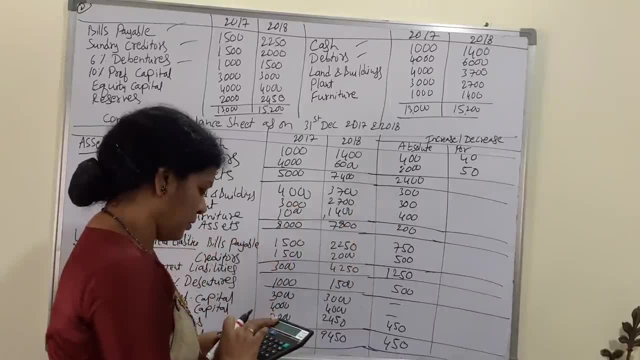 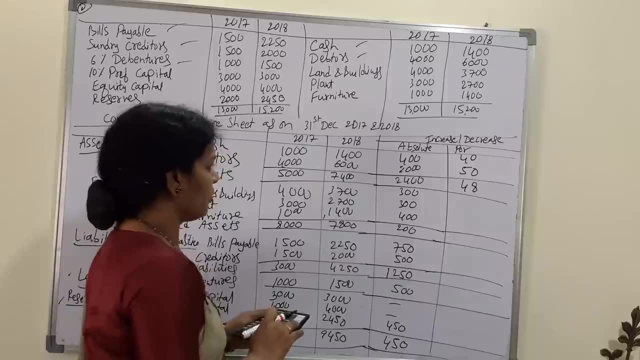 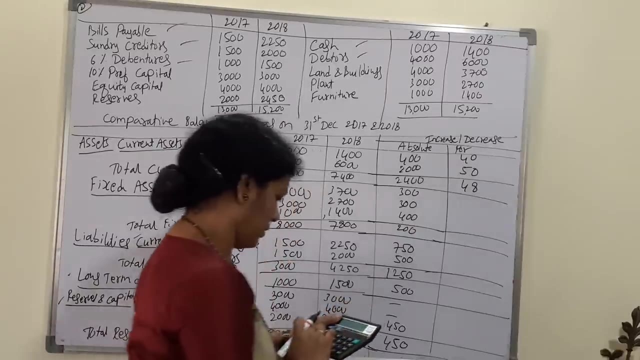 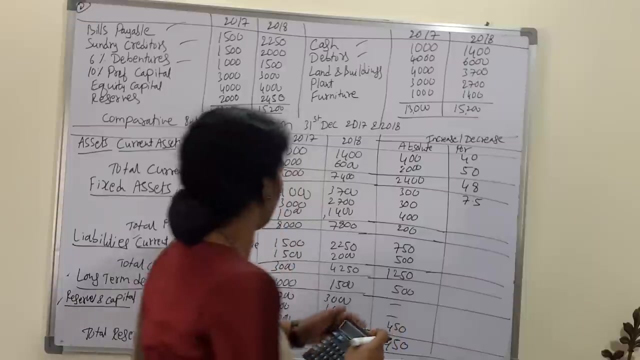 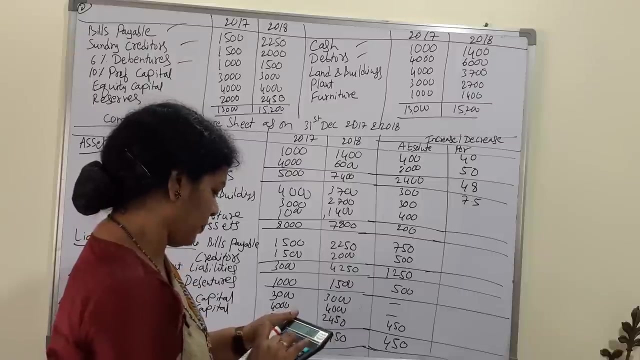 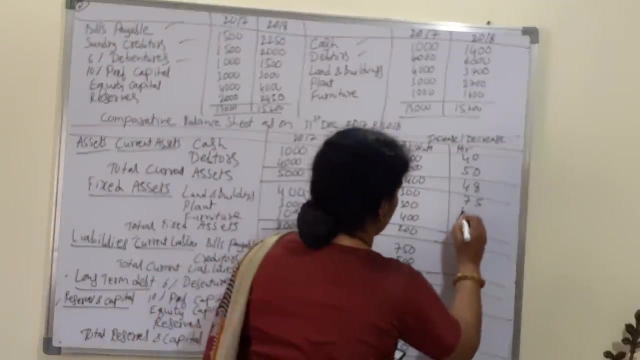 to two thousand four hundred divided by 5000 into 148%. next 300 divided by 4000. 300 divided by 4000 into 100 to 7.5%, next 3000 divided by 300. 300 divided by 3000 into 100. this is, this is 10%, next to 400. 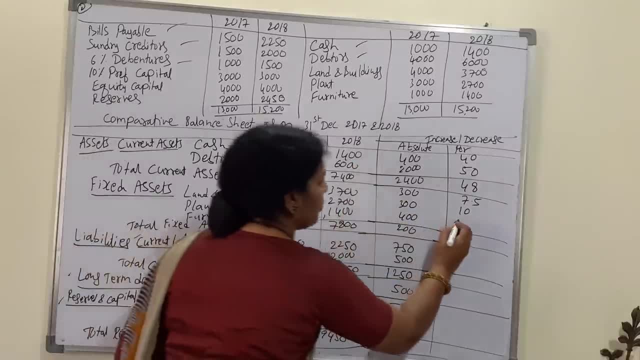 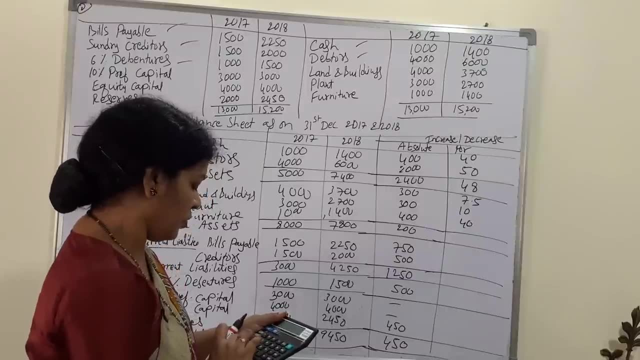 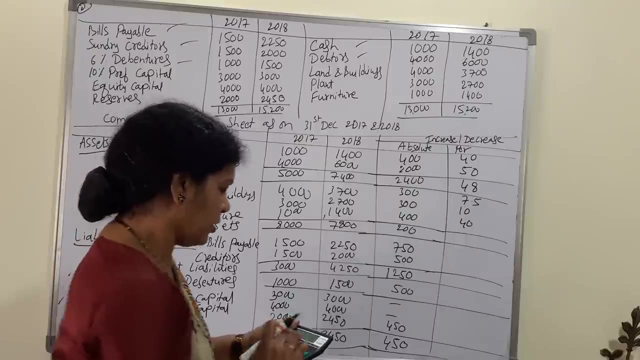 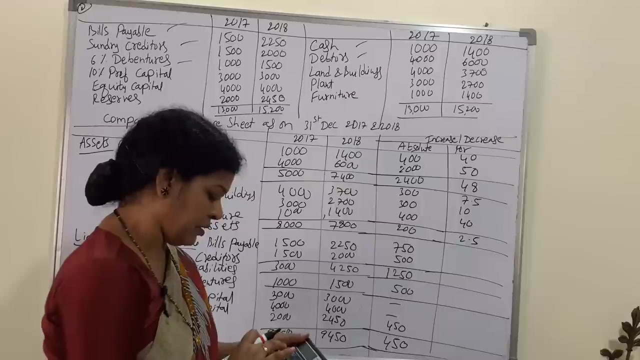 divided by thousand. already we have done a, so in 40%, it is the same one. next, 200 divided by 8000, 200 divided by 8000 into 100, it is 2.5 percent, in the same as 750 divided by 1500. 750 divided by 1500 into 100 it. 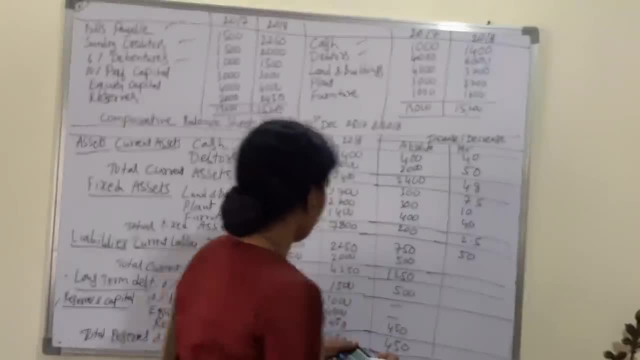 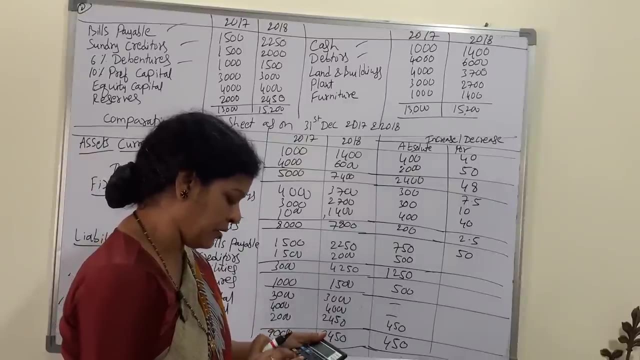 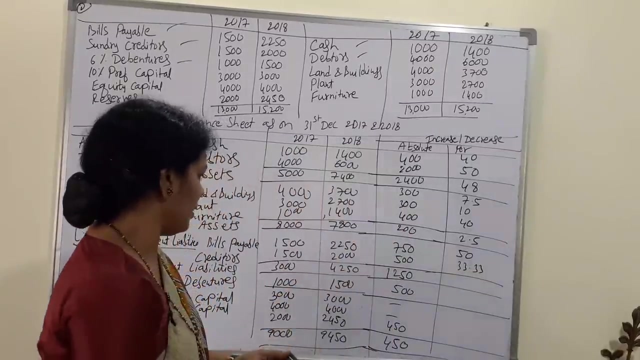 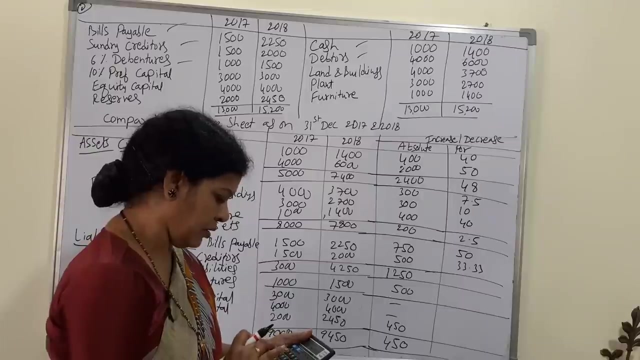 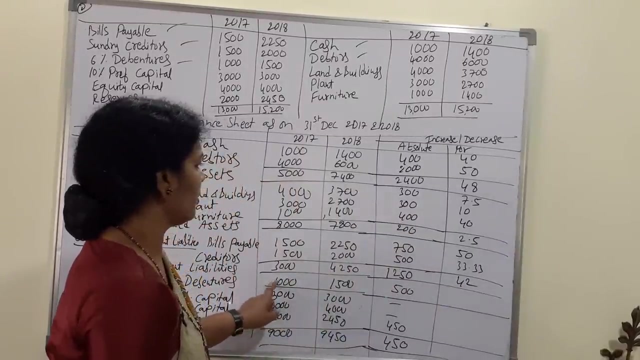 comes to 50%. 500 divided by 5: 1500. 500 divided by 1500 into 100, it is 33.33. next, 1250 divided by 3000 into 100, it comes to 42 percent. next, 500 divided by thousand. 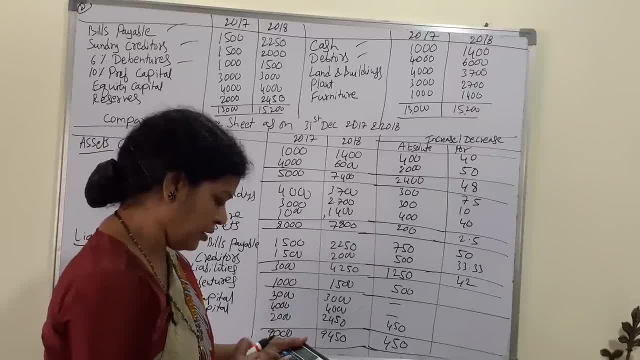 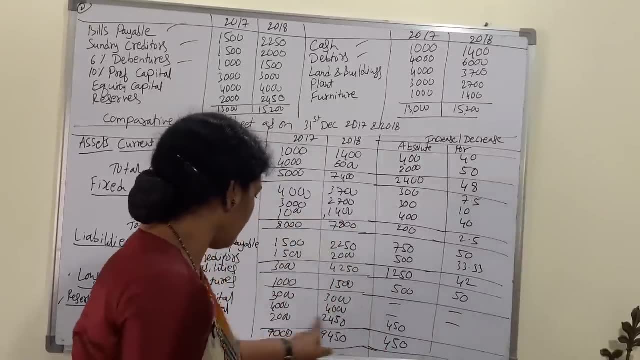 into 100, comes to 50 percent, and these two are nothing. is there? next 450 divided by 2,000: 22.5. next 450 divided by 9,000น. next 450 divided by 4,000: 9000. forget second phrase. 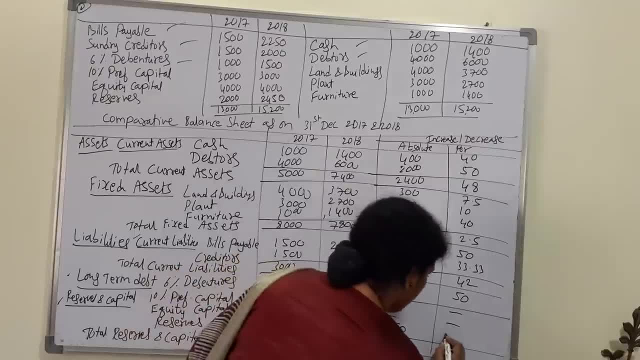 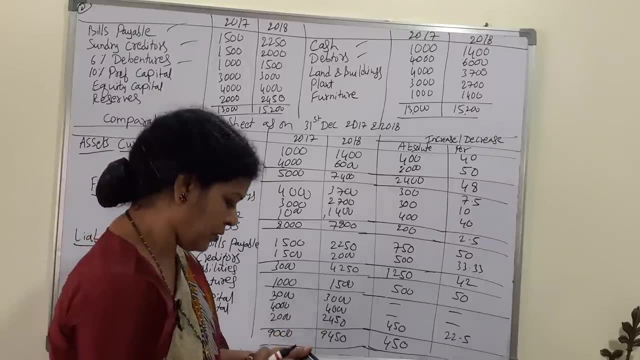 first paragraph, let the next order of minus 52.5. can you see the same? taking the in of the power is right. the verdad work that we recorded to thiscore, 1th in 2.5, until what is wrong in N 1-4.5. 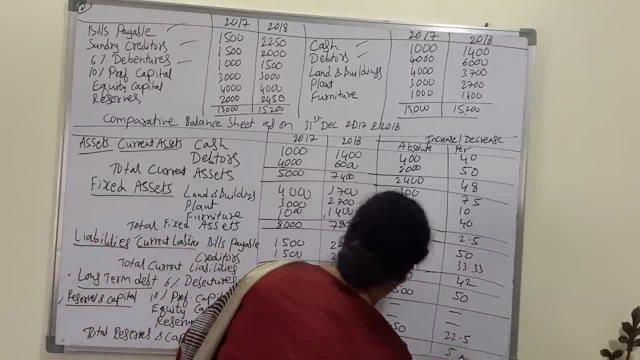 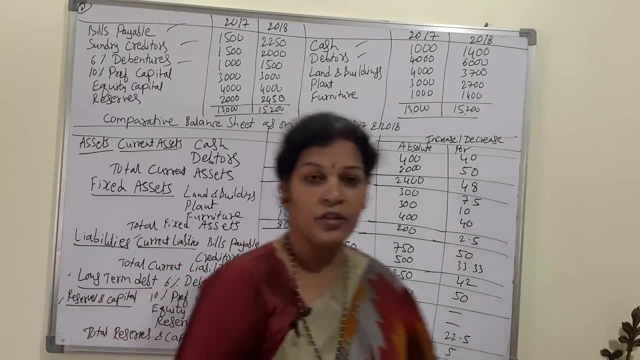 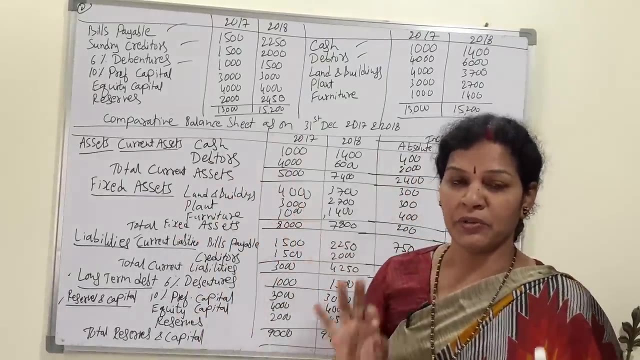 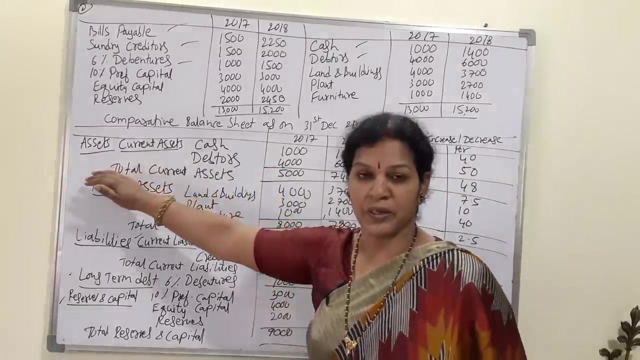 200, it comes to 5%. so that's it. so calculation, this, everything is just calculation. only you need to understand is this part and how to calculate. let me give you a recap. balance sheet is simple where comparative balance sheet is simple, only performer. you have to follow as I have done. assets we are taking. 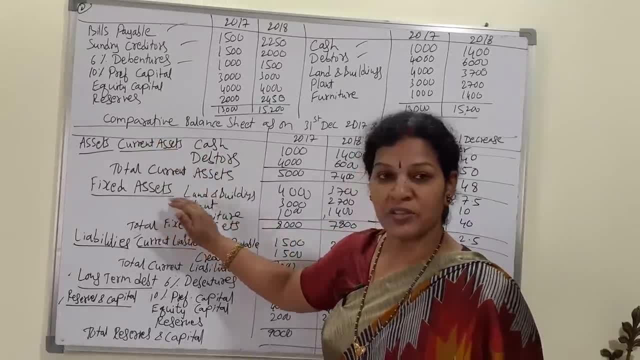 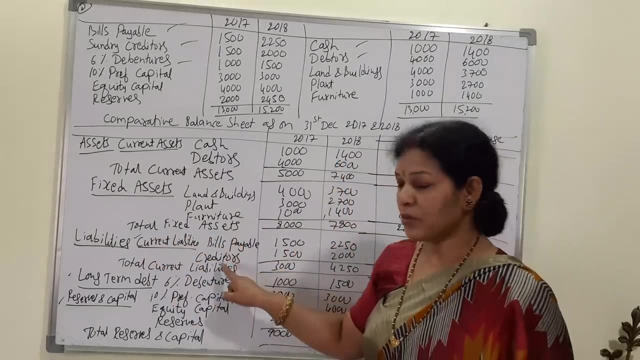 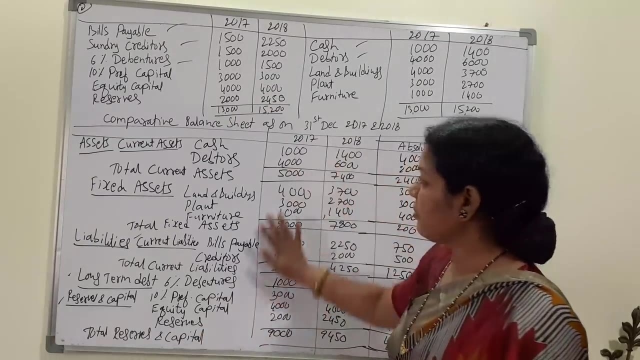 current assets identified and written over there. then fixed assets also identified and written: total current assets, total fixed assets. then after that, liabilities- current liabilities, total current liabilities, long-term debt and reserves and capital. three total reserves and capital. so this performer we have prepared and increasing or decreasing that we have written. 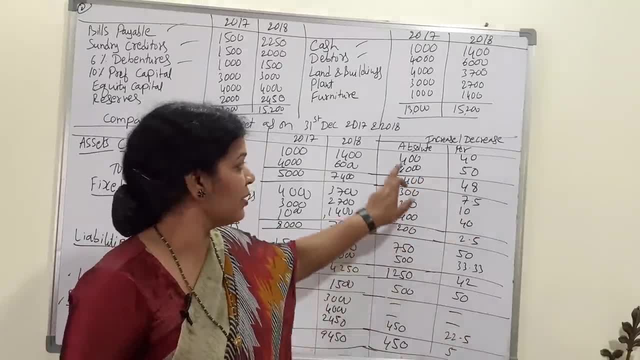 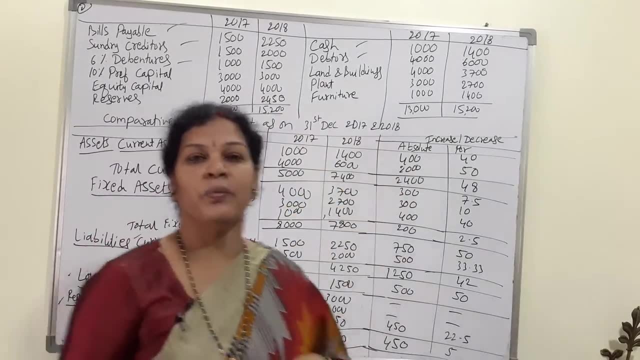 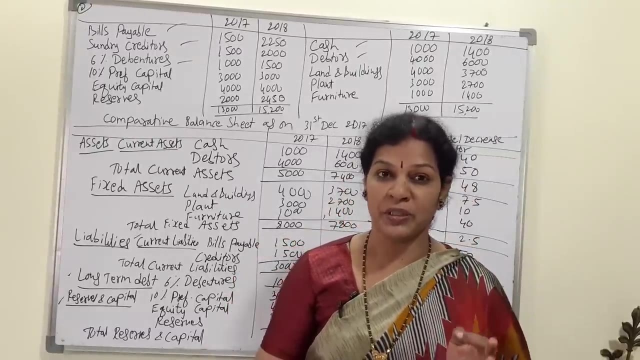 percentage, always percentage. you can calculate like: so, whatever is increasing or decreasing this divided by the base into hundred. so like you've got everything. now what to do? just to. preparation of comparative balance sheet is not complete. you have to give the interpretation of this. what is this interpretation? how we can give so you? 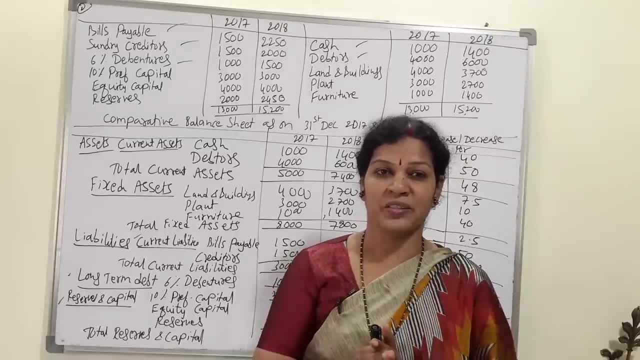 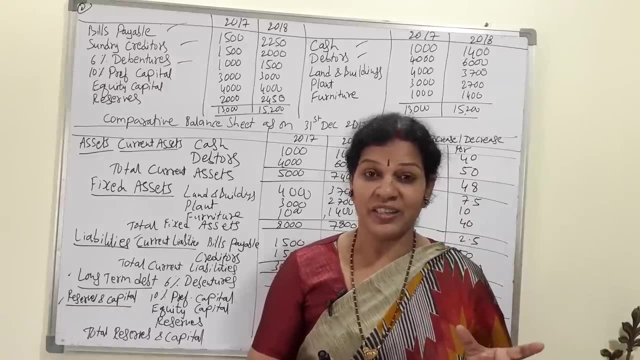 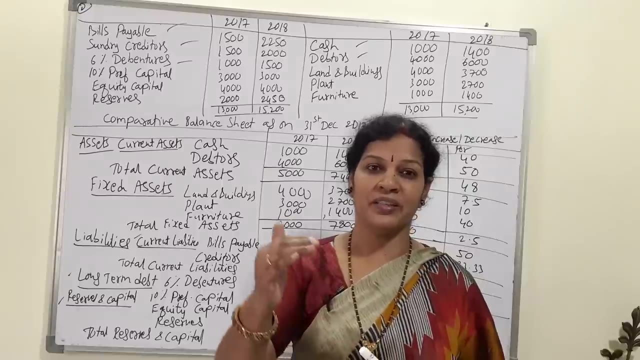 can compare it from current assets to current assets. how much is increase fixed assets so much increased? what does it mean? you must know, first of all, if current assets are increasing means it's a good sign current liabilities are increasing. but if you compare it with current assets and current liabilities, 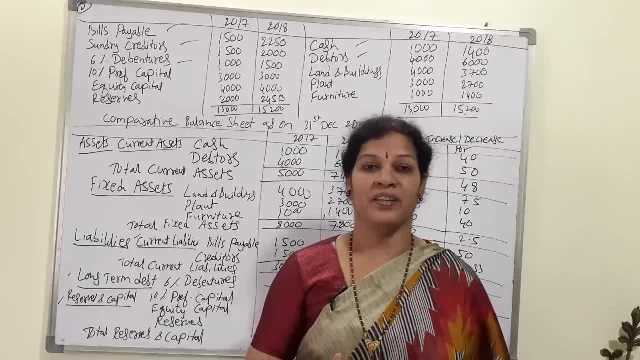 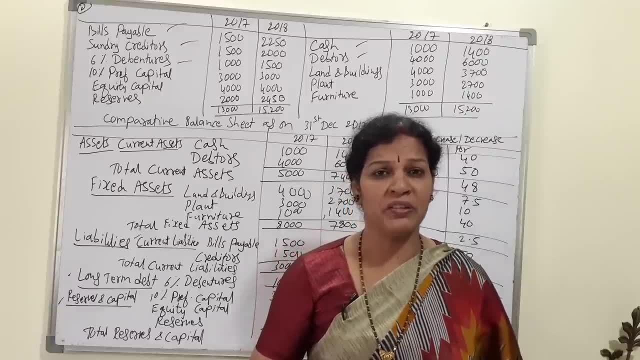 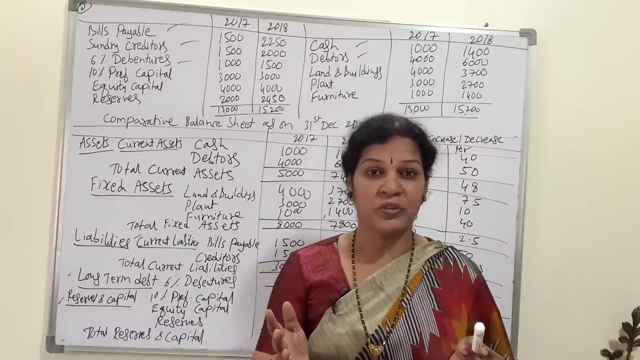 current liabilities increase should be less and reserves are increasing. it's a good sign for the organization. reserves means from where do we provide reserves? reserves are from the profits of the last year, last year. if we get a lot of profits- total profits- we are not going to share it to the shareholders, or total profits we are not going to enjoy some. 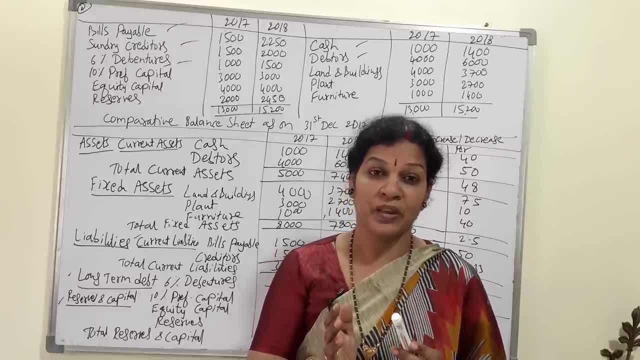 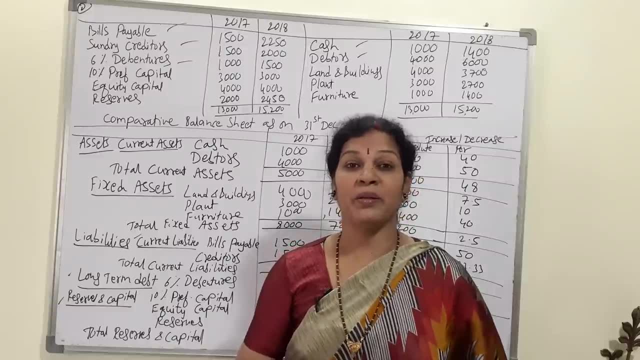 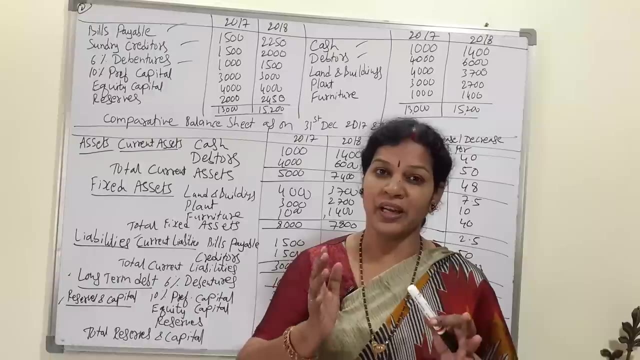 of the some percentage of the profits will be transferring into the reserves. reserve is increasing means it's a good sign. so like and in the same way capital also. capital is increasing means business is expanding. so in that way, each and every transaction, every item, you can take and you can give. 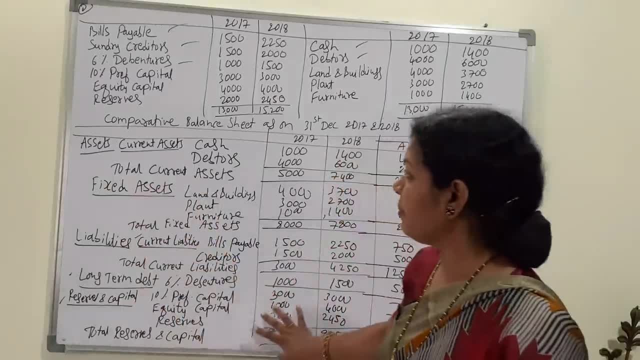 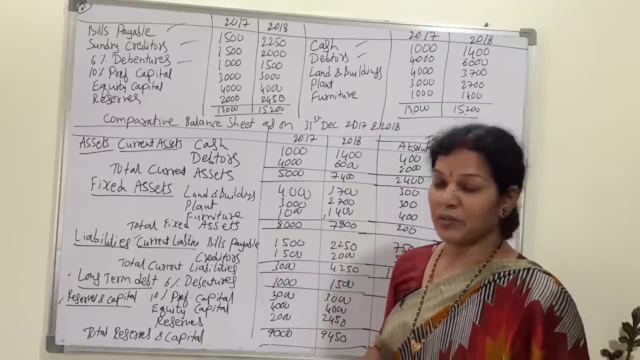 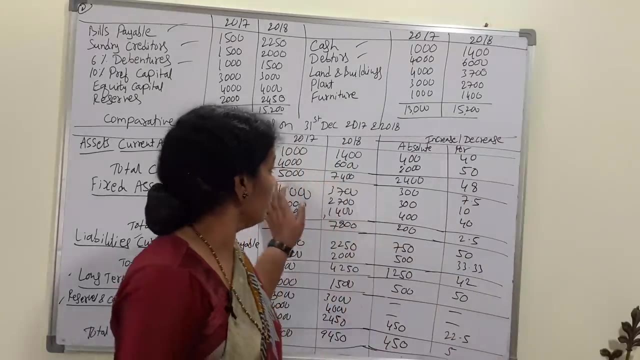 explanation how, for example, same problem will see. so after this problem, we have to keep sighted interpretation, point number one, what we can give, point number one. so here, total current assets: current assets are five thousand to seven thousand four hundred. it's increasing current assets. always increasing means financial position. 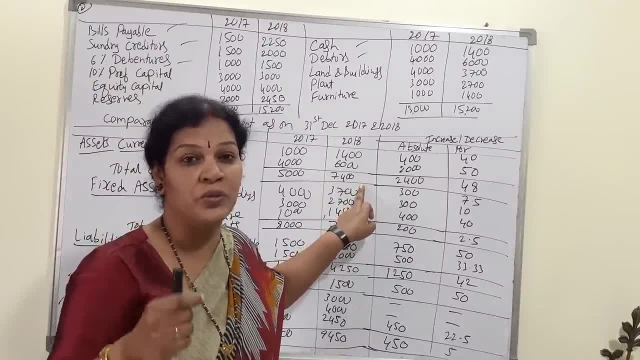 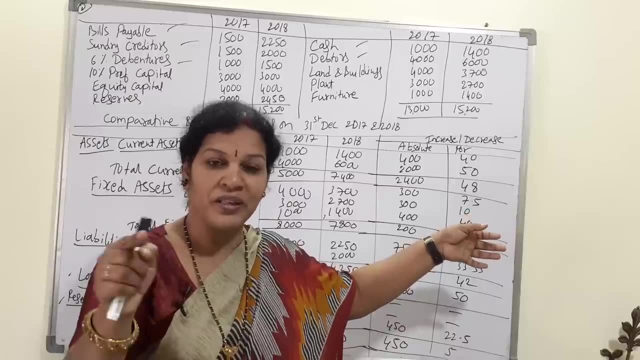 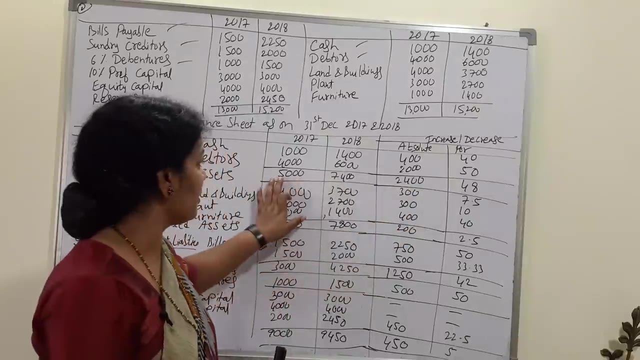 liquidity financial position of the organization is good. how much it is increasing? forty eight percent, almost fifty percent it is. so first point: you can write: current assets are increasing by forty eight percent. or you can say: current assets are increasing from five thousand to seven thousand four hundred. 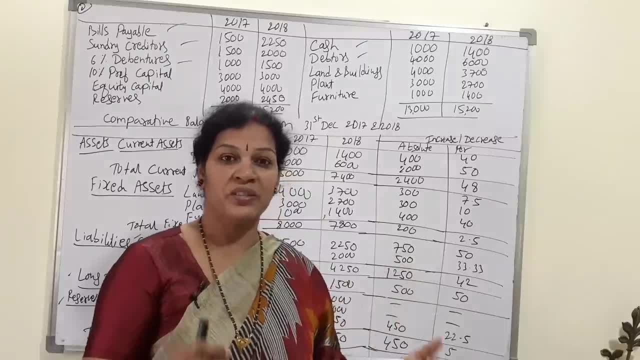 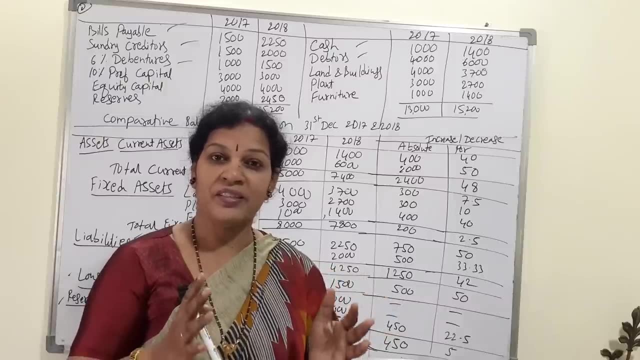 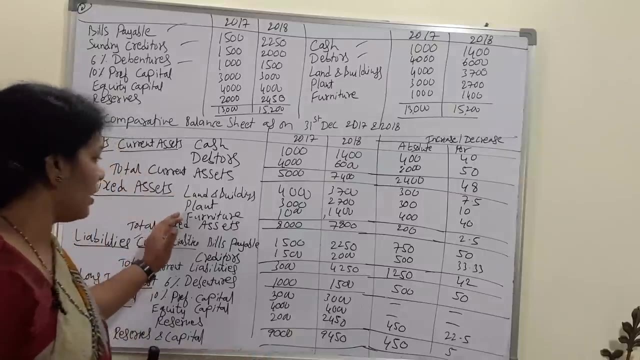 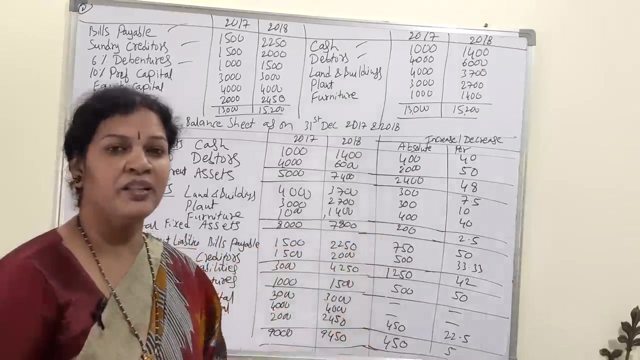 that is forty eight percent, which is a very good sign. liquidity position or financial liquidity position of the organization is quite good. hence we can say the organization is in a good position. first point number one. next, take the fixed assets. fixed assets are here increasing. it's a little bit decreased, it doesn't matter. regarding the fixed assets, we 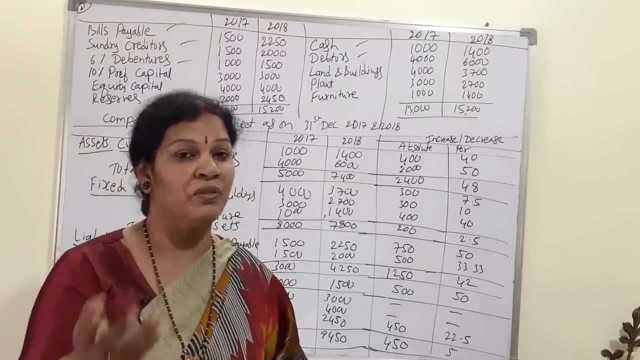 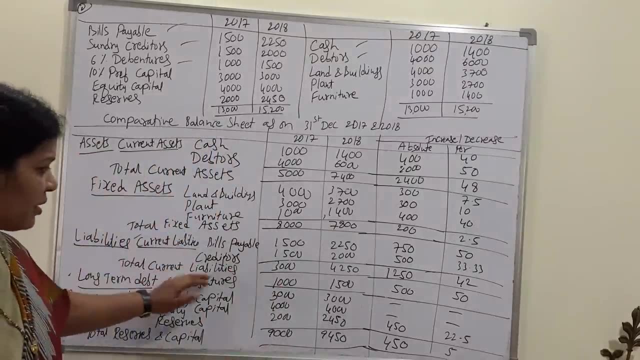 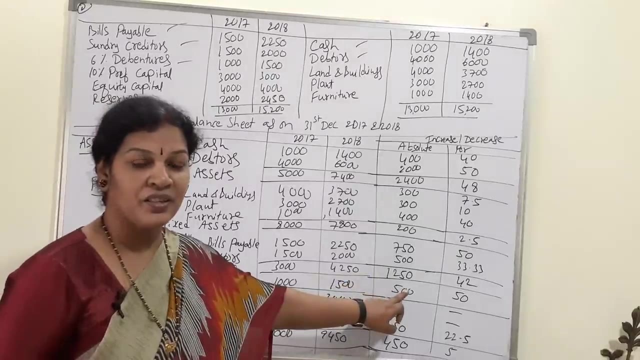 can't say anything as per the requirement, will be purchasing or will be selling. so, regarding that, we need not to give much interpretation. now, coming to the current liabilities. current liabilities total are 3000 to 4250. this is also increased. current liability increased. how much? 42% it is increased. 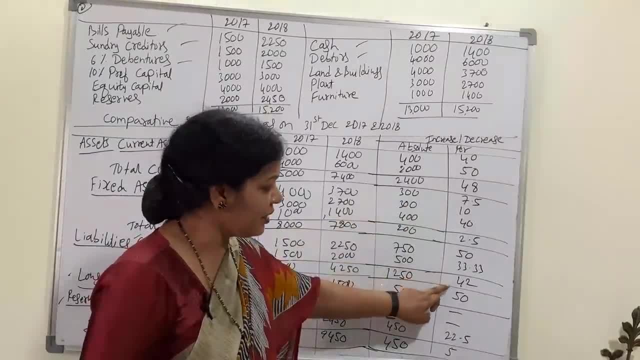 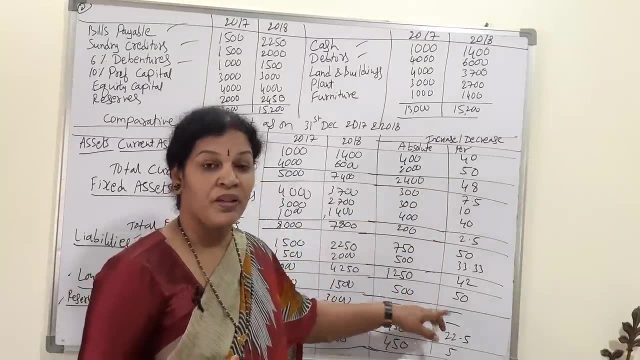 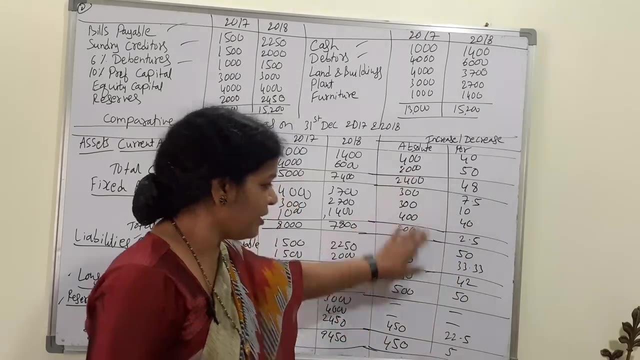 but whereas comparing with the current assets, current liabilities are increasing by 42 less less than the current assets. 48 percent means the company is in a position to pay the current liabilities from the current assets. like second point, you can do this. and third point is that long term debentures, debentures, are here. it's. 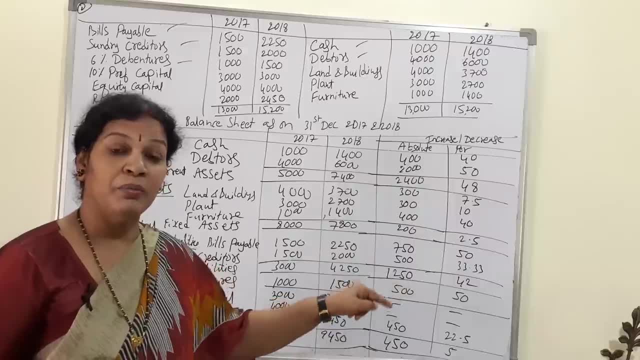 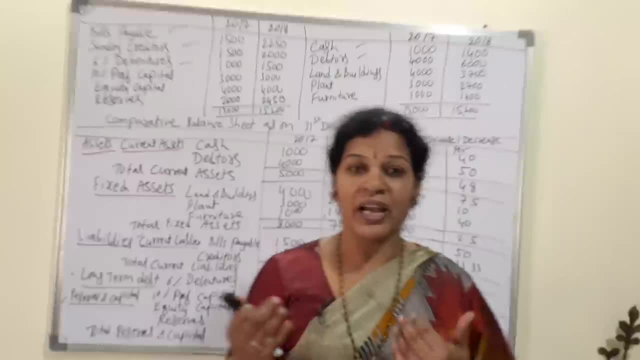 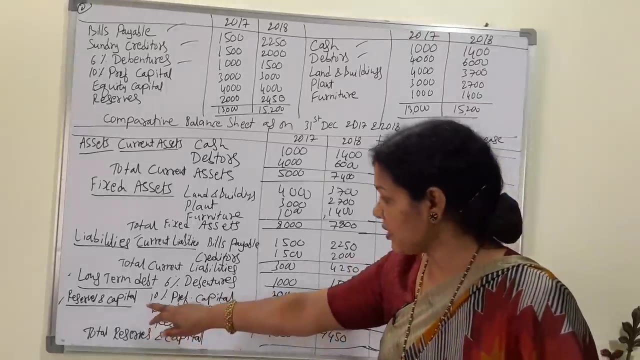 increasing 50%. increased debentures are increasing means it's a very good sign for the organization. long term debts we are increasing. increasing means we are having much, much of the funds. so this is also very good sign. and last point, which you can take: reserves. 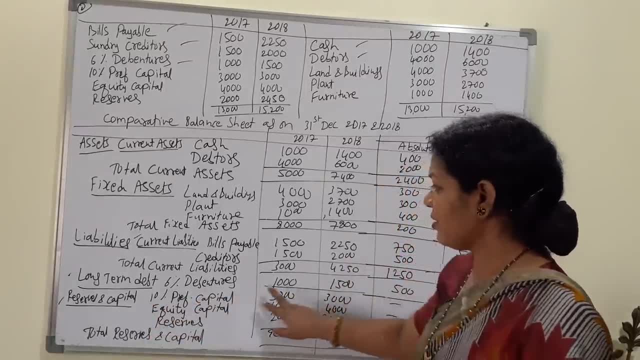 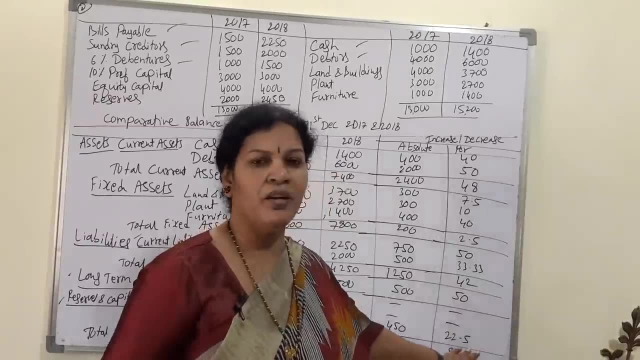 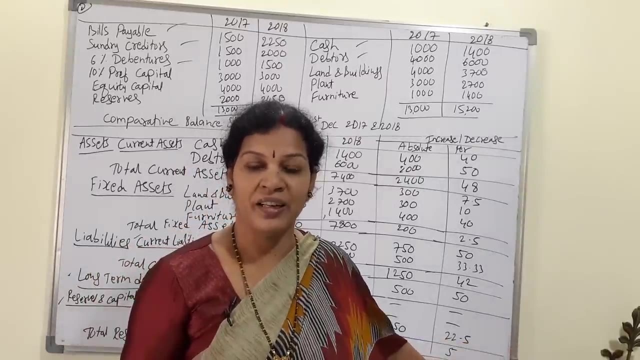 preferences share capital. there is no increase or decrease in the prefer pursue capital and equity share capital, but reserves are increasing by 22.5 percent. anyway. it's not high amount: 50%, 3 parcel, 40 percent. it's a very good sign, but anyway, reserves are there. not only it's there, it's increasing by 22.5, 22.5. 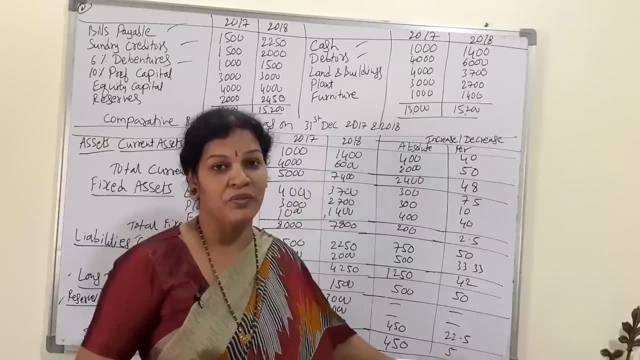 percent. so this is also very good sign for the organization. like point 201, point number 2, like give the interpretation. and last but not least, are year 10 to 201 lie convenient? I can give you any rupees to the project. you can give me any advance note. 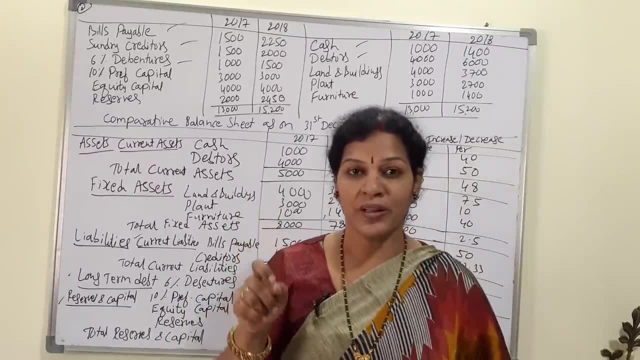 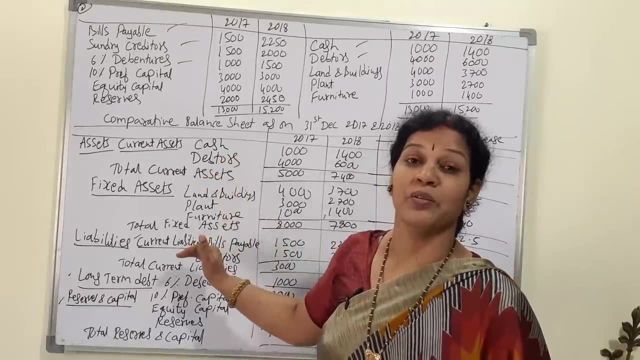 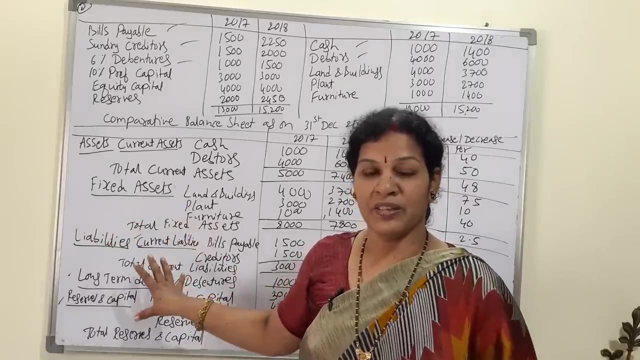 And lastly, last point, you can say overall the company's financial position is satisfactory because current assets are good. current liabilities are also increasing. but comparing with the current assets, current liabilities are decreasing less and also company's financial reserves are increasing and also debentures are increasing.